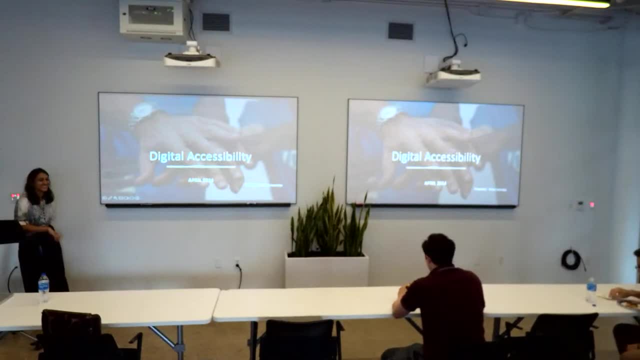 And five: Yeah, So it was a good event. It was a good event, But they would like to partner with us. We are partners, So automation will run on the actual mobile devices. But soon we will be hosting one of the events. 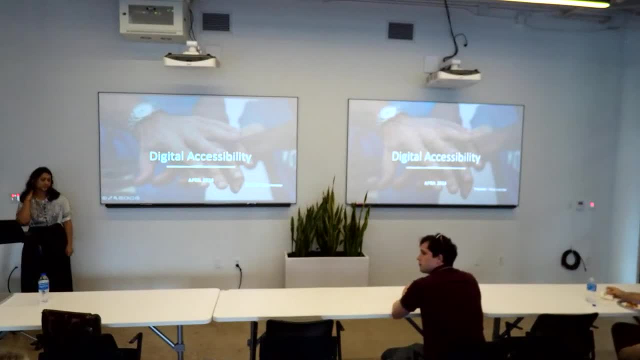 Yeah, No, they are in India, But they have presence. They are in the relation to India and Japan. So, yeah, they have good presence in India And they have good customers. Yeah, Yeah, Hello everyone, Hi, Yeah. 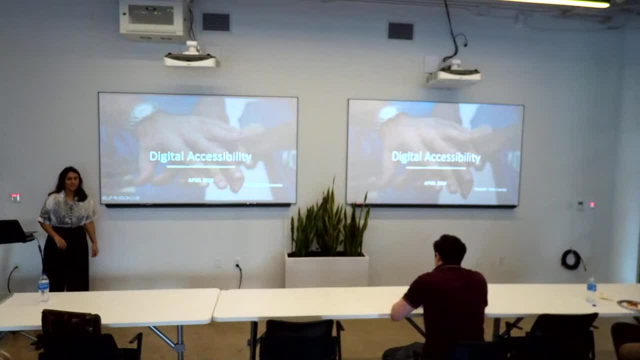 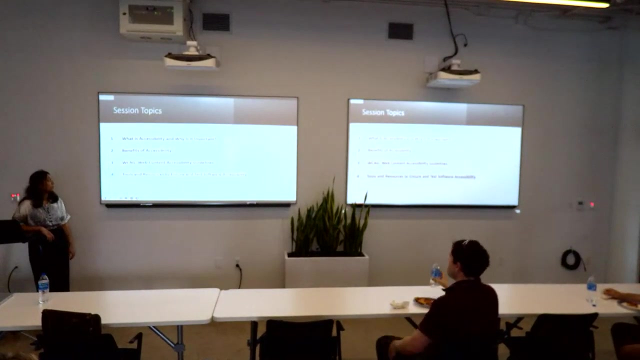 Yeah, Yeah, Yeah, Yeah, Yeah, Yeah, Okay, Yeah, Yeah. What are the benefits of the SPV, What are the guidelines to follow to make the SPV look better in the future or not And, last but not least, what are the benefits of the SPV? 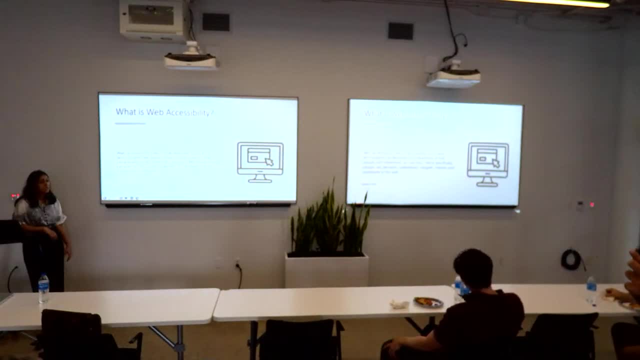 So what we are going to talk about. what is the SPV? In a simple language, I would say: design and the adoption of the SPV is a very, very important part of the SPV. So the main purpose of the SPV is to promote equal opportunity and anything with discrimination. 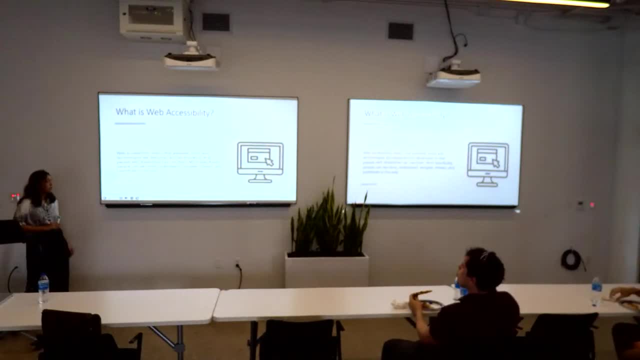 might provide equal rights and benefits for the population. Why should we care about So? according to the SPV, there is a 15% of the population who is studying at a SPV. It's a line, It's a large number. 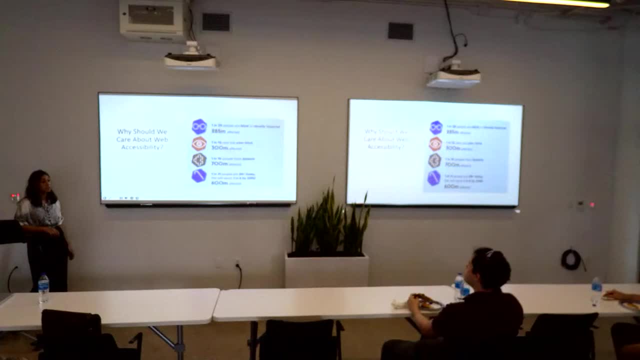 And according to the SPV, there is a 15% of the population who is studying at a SPV. So in this particular world, we are providing the SPV to the people who can't attend, who don't have on-road, indoor and internet access. 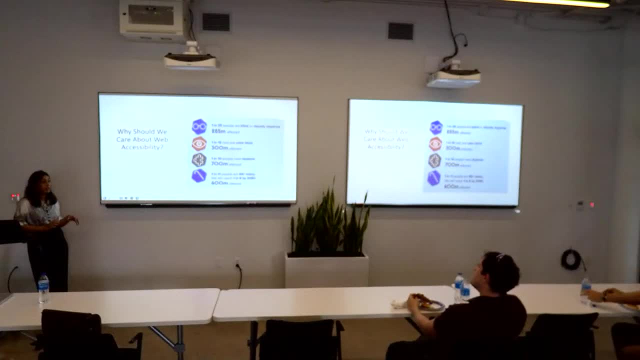 And when people try to come to our website and try to use our website to access the technology- access the technology not to put all the information to the end user- they can't do it, So that's why we care about the SPV. 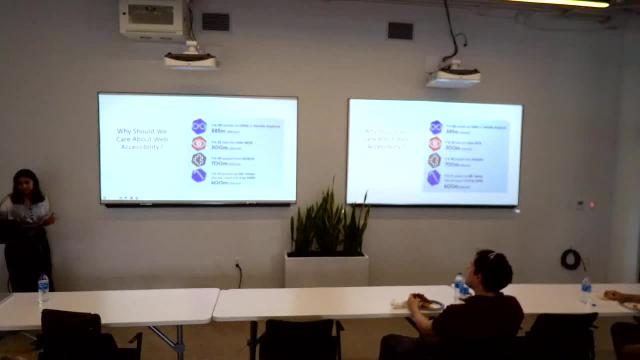 There are some things that you can see that are permanent. There are some things that you can see that are temporary. There are some things that you can see that are in situational. For example, here we have one hand that is in situational disability. 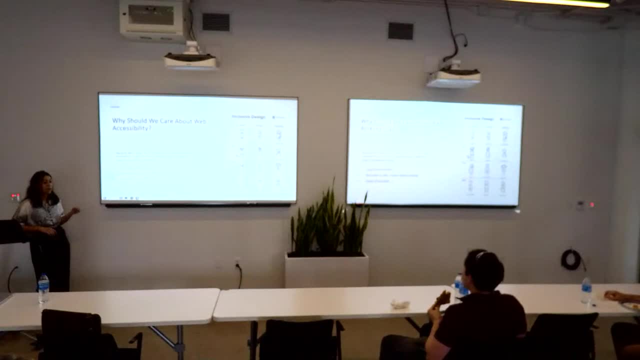 Or if you are in an out-of-town environment- here that's in situational disability. So we can provide some of those things. If you are in a situation where you are going to a community of people who are at different places at different time, that means you have a separate person at different time. 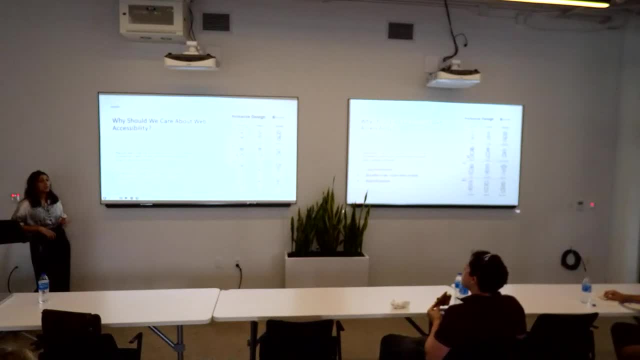 They can be easily separated. You may also be able to connect with them. These are like temporary situations, And in a non-neutral situation they can be even turned into temporary situations. But there are some other things that we are talking about: self-sufficiency and self-reliance. 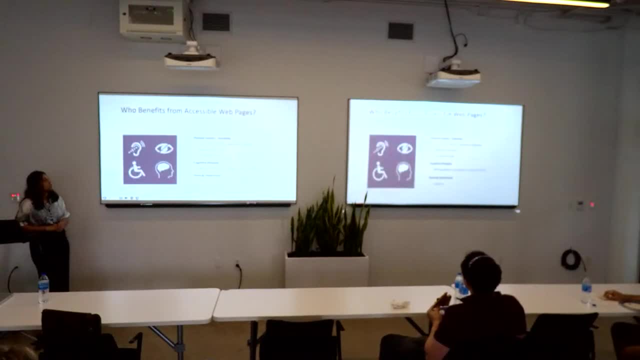 So this one is a very important thing. So we can provide the SPV to the people who can come to us, and then the person can go and attend our Badg for therapy. So this is a very important component of a healthy life. 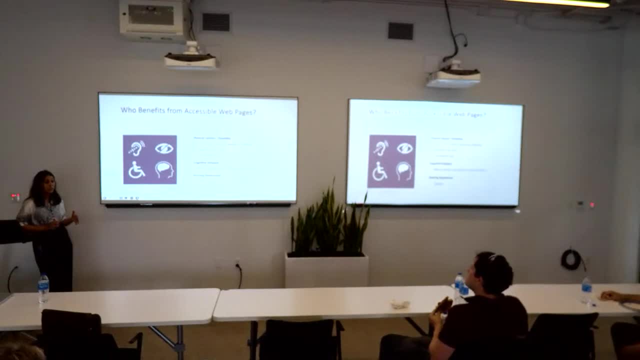 And this is a very important component of a healthy life. they have to rely on the keyboard, so they have to be able to voice the message. So if you provide a web frontend accessible, they can access the web frontend. If you provide a web frontend, that is easier and less time consuming. 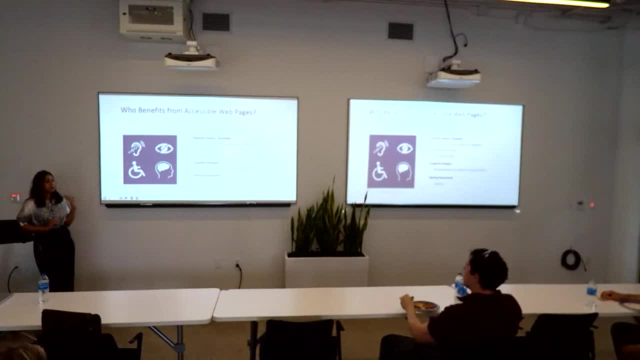 you can provide the proper instructions, you can provide the help, or if you provide a web application, then you can provide a web application People who have to be clear in this area. so if there is audio and video, if you provide a web content that is introverted to caption. 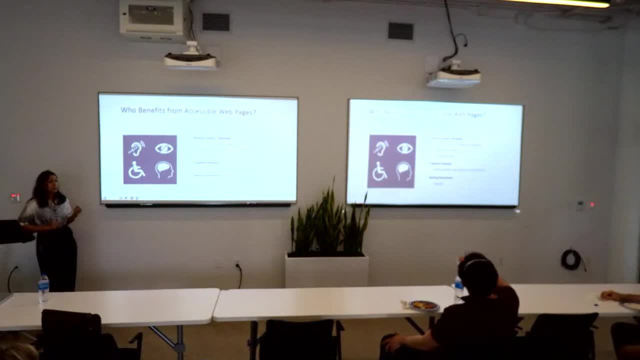 or audio content that is introverted to landing. so if people cannot hear, then they have to use the web frontend and use audio to provide information People who have the low vision. so if our web content can zoom out around 2 percent, 200 percent, 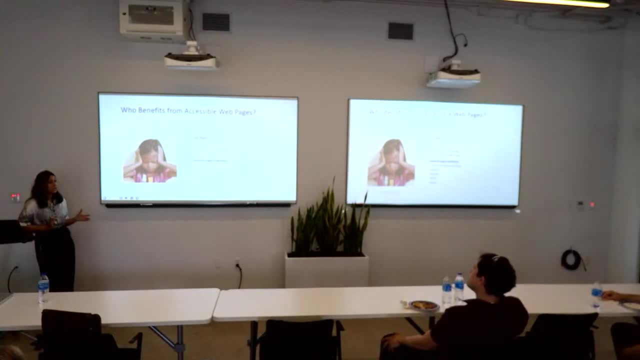 and if the web content doesn't work functionally. so if I provide information in the web frontend, then the people who have low vision can also access the web application. People who have a neurological disability: when people have a neurological disability, then they have a more focus on their attention. 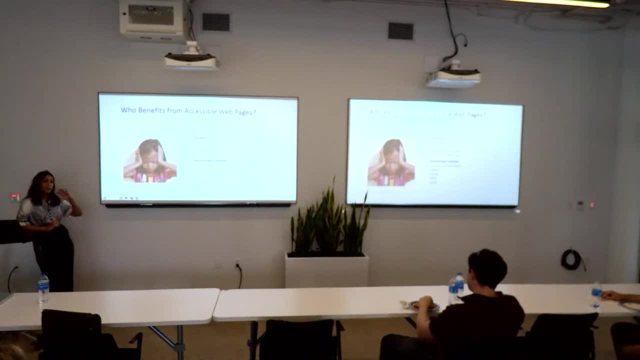 So there are many ways of education, like advertising. there are many ways of putting on, like I said, putting on web specials. so we should use the power to either take a high or take a lower level object so they can focus on the actual web content. 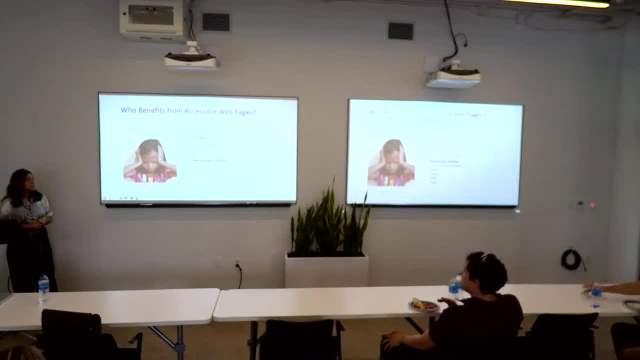 So this is our web presentation form. I think it will be time for all of these people to be interested in accessing the web content. What are the benefits of having the application? So definitely we can teach how to pass it on to people. 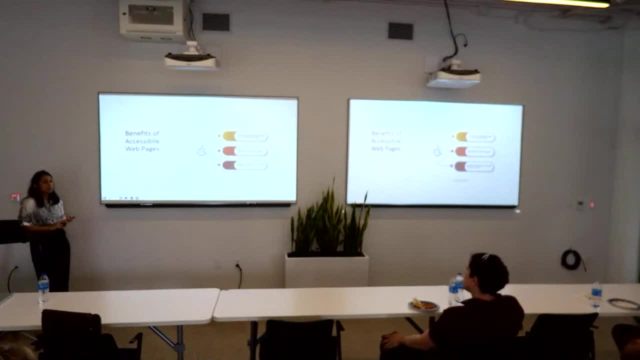 as well as you. with this type of web content, you can be useful, In fact. I have a few questions for you. Can you tell us a little bit about an application? Can you tell us what kind of application? So what kind of application can the user use? 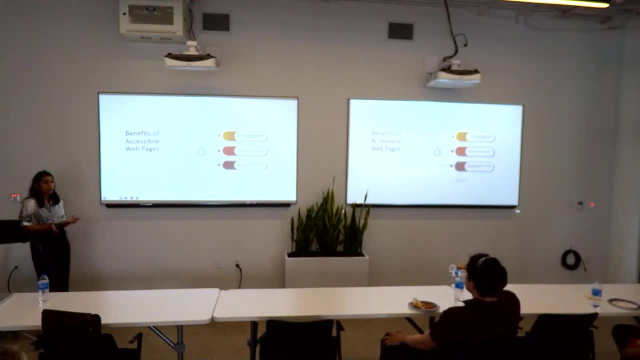 If you have a web application, if you have a browser, which is a browser, and you have an application, What are the benefits of having the application? We look at the information given to us. I have an application that they can see. 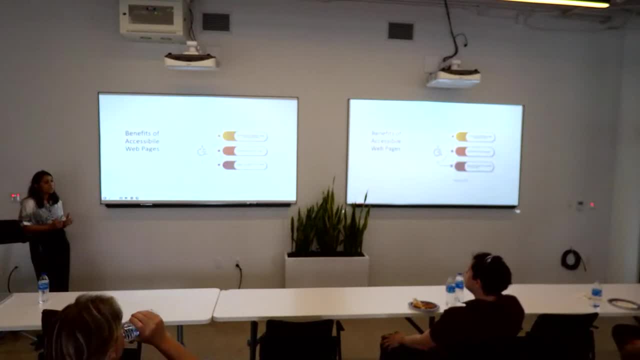 and when they see this they have to send a request for a that application. How can our client access it? There are many fortunate 500 doctors that have worked with us because they didn't make sure that there was a common quality in treatment, so we want to make sure that people get regular. 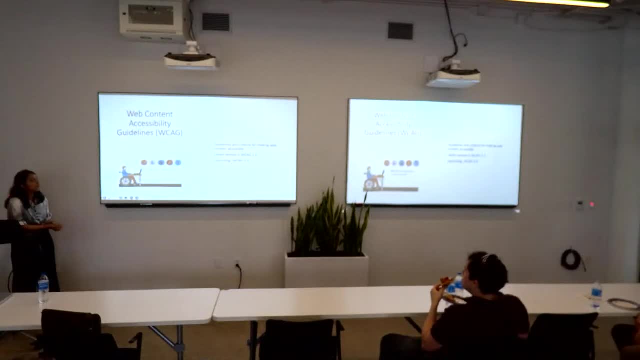 care. We are trying to make sure that people get regular care and we are trying to make sure that you know people are coming to us for treatment, for treatment, and the quality is great. So what is? a lot of success stories happening. see, they have done I can. I can give you. 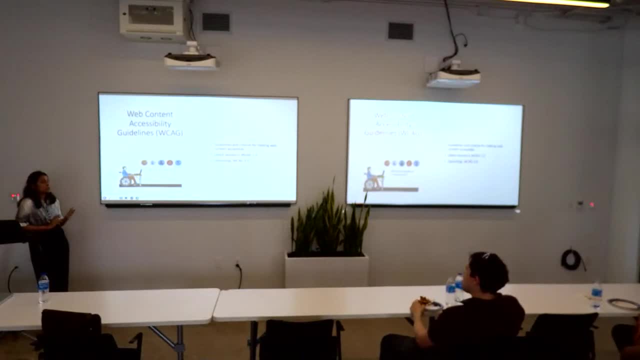 all the information I can give you. It's a lot of success stories happening. What happens is they make sure that patients who are tired after treatment is okay, they are not tired. they are not tired after treatment, right? So I think one of the group of students is the latest, but I think one of the most important. 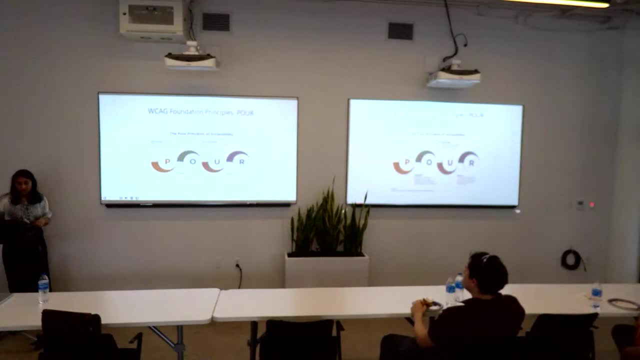 students are coming out today We just have the four foundation principles, or the four principles: P stands for the participle, O stands for the operable, U stands for the understandable and R stands for the cooperative. So participle. there are many people who take participle to be our peer to the polytechnic. 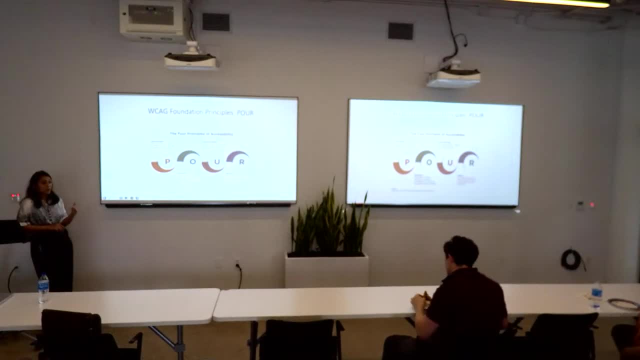 peers. So if I am on the internet I cannot see the screen, so I have to be able to access the technology. So we have to forward our design of our website in a way so that we can get all the important content and we can transfer it. 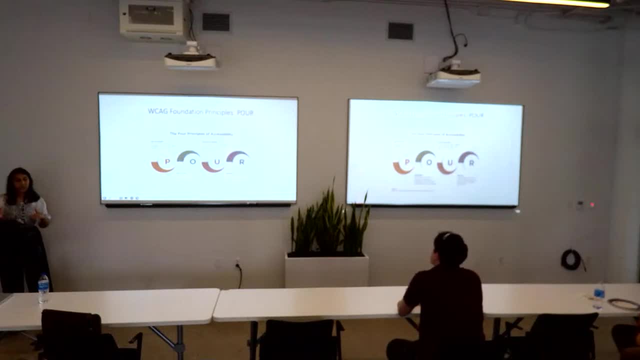 And through the access to technology we can transfer all the content we need and see them, So you know. so information is personal. If I cannot see it, if I can't see it, I cannot see it And I cannot see it. 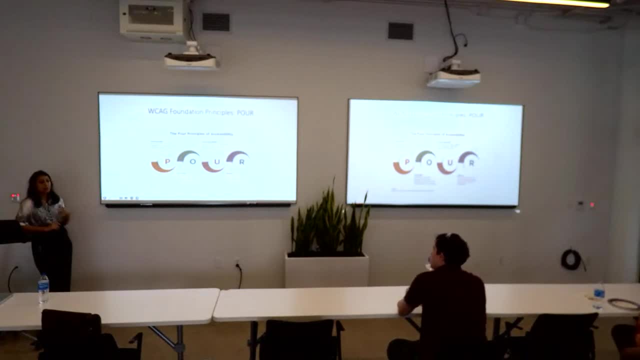 But, peer, we can provide it over. we can't get our answer over and it can't go. and then multiple people: we can provide the label so any of them know who they want. So that's all another part of the label. 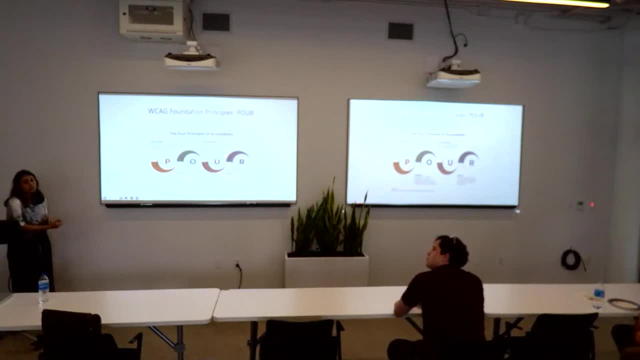 For the undertand, for office. there are many functionalities in the dual email, such as the way you have the button. you can have the ring go horizontally, go vertically, go forward, backward, go backwards. so if people who are starting to come out, we should provide all the operations and 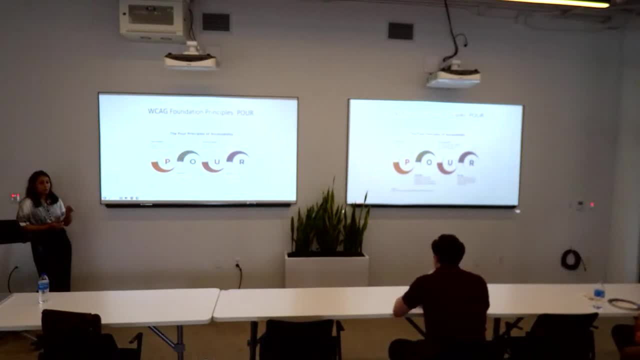 operations to be done in the next water. If there is an air leak, the sensor should get to load. the sensor should be moving one by one hour. it's not a single air leak. the sensor should never go to the back way. 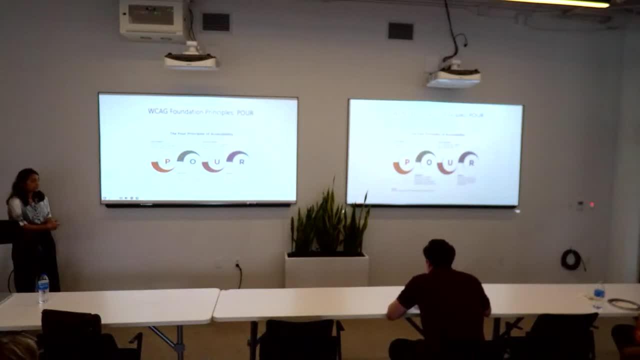 so all the functionalities should be possible right now. Understandable: we should provide a proper label name so people know what kind of data- input data- they need to go to the particular input field. so those are the understandables. Robust: there are many web applications. they work totally fine in the probe but other 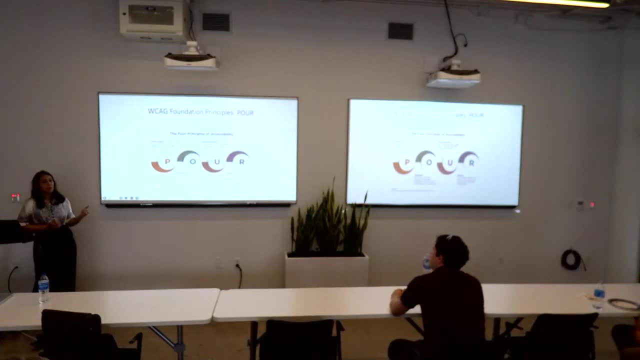 products are far too far, so we have to make them work in a way that they work totally fine in the all of the algorithms. There are many web applications that work totally fine in the desktop. The desktop doesn't work too well. some web applications work much better than others. 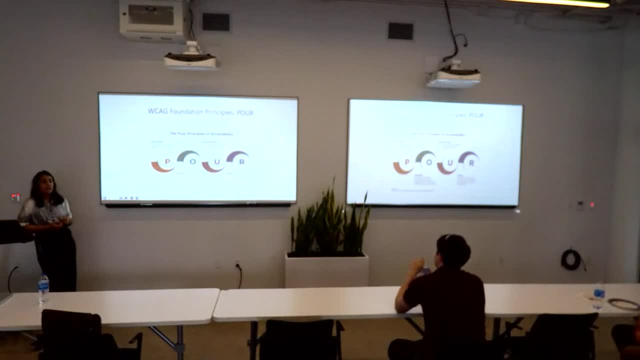 in the desktop, like, for example, if you want to allow a zoom in for 200% of the data, you cannot see the data. but if you want to zoom in for 200% of the data, so those kind of issues shouldn't happen in the web application, so it's a quality problem. 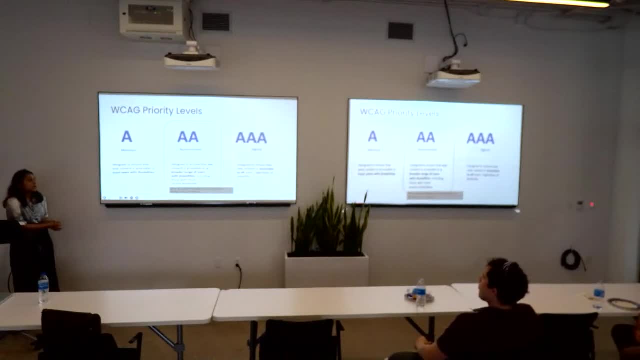 Here are the sub-subjects we take priority labels: label A, number A and number A. A is the minimum label of the system. A is the minimum label of the platform when you are building a web content or if it is. 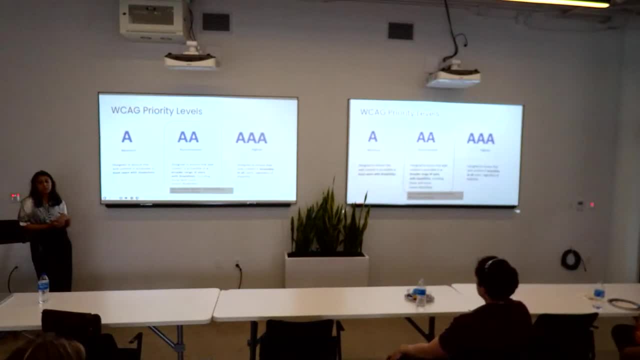 a bootstrap, you can stack the label A up when you are building a web content in the label A. that means you have to remove the city, but it doesn't remove all the city, but you are at a good position. so what, what? what are the label A having the text alternative? 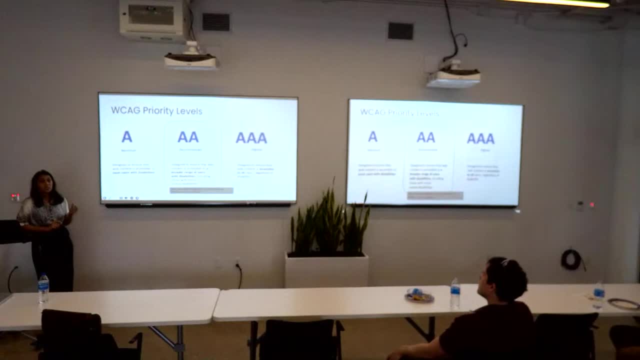 for meaningful information. meaningful information means the image has to be not the same. the image has to be the same: The context. if you do not provide that context to the user, they might lose that context. So that's for us, that's for the users, so for the people in the institution to provide. 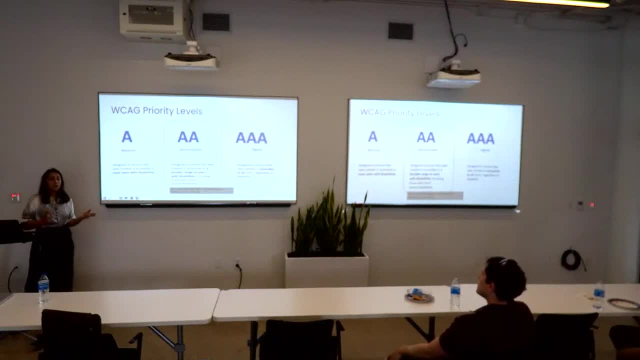 alternative text. for example, if we have a building or a facility or a customer service and the users say, hey, that's the technology that we want to have, and user want to know that what they do has to be the same, they want to know what the system is doing. 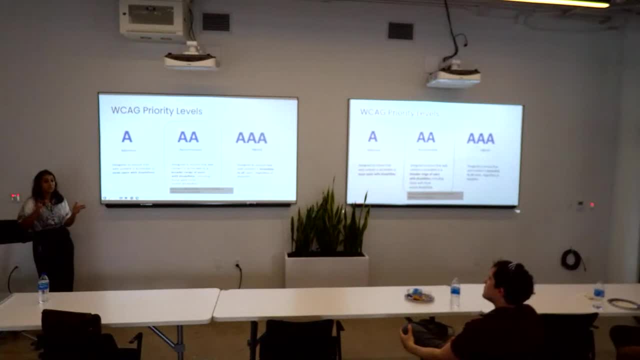 So we have to provide alternative text to the person, even if the person doesn't know what the system is doing. we have to provide that so the user can know that what the system is doing. Another thing that falls under the label A, that means again, a web content should be: 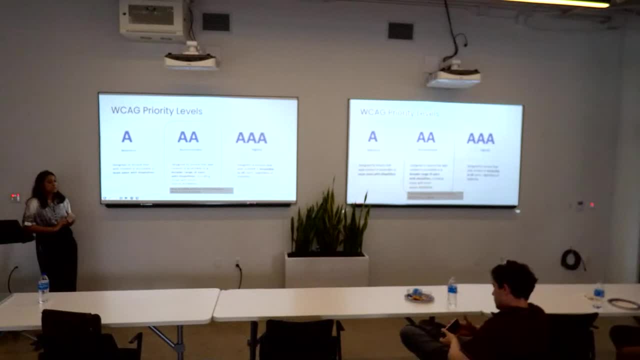 more accessible. and another thing that falls under the label A is the production we want to get from the user, because when you put the password, the border of the password is different. what if I have a current language of the same name? I'm not sure to know if. 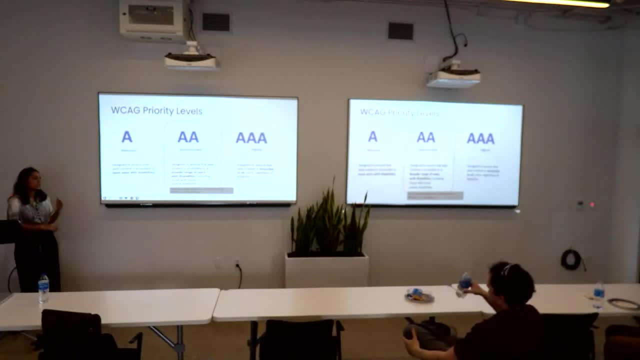 this is the piece that I'm trying to get right, So there can be that type of issue. so when the proper error metering, proper icon, that indicates that there is something wrong with the password. So those are the criteria for accessible level A. 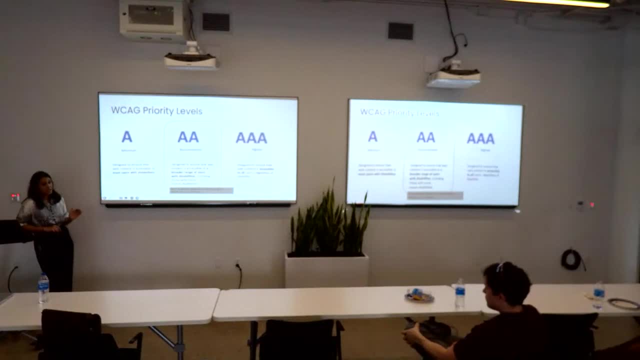 Now level A. so once you achieve the level A successful criteria then you can start to work on level A successful criteria. Level A is the most common, level A is federal and then level A is agency. but to follow the level A you have to have a level A successful criteria. 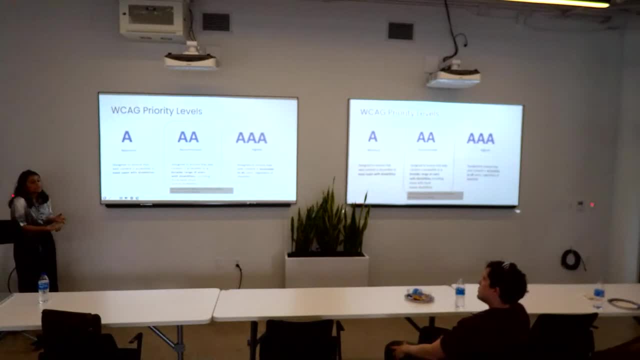 So what falls under the label? the level A- successful criteria users should have the functional users should have a degree of 200% without using any functionality. There should be consistency for the page. if you have a web page, then you search bar. 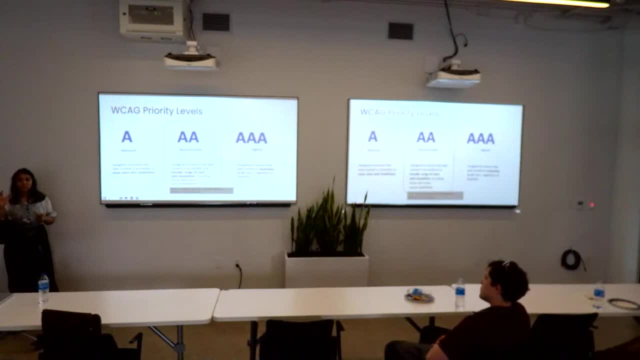 on one page and not having the search bar on another page. that is not consistent. that means your web content is not as successful as the other. let's look at another example of what we did. So in this image we have a button on the scratches, so on the other foot, the button. 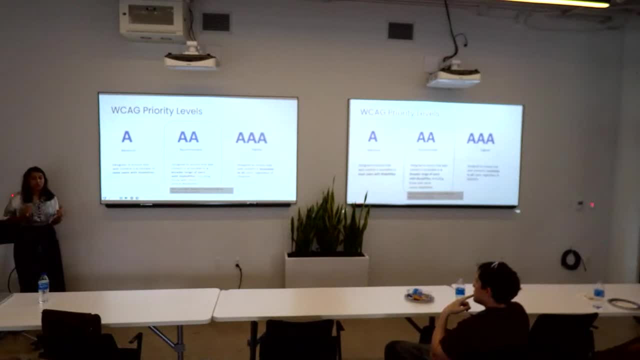 is in the bar, so deserve to have the. any accessibility for them. it should not be managed, because each page they have to search the your web content more so for them it is too much, so you have to make sure about their proper instance of consistency there. 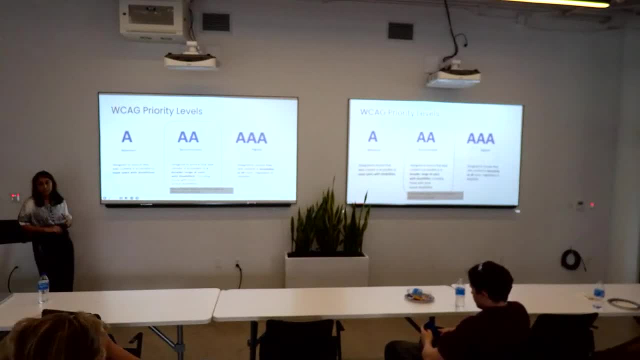 should be more than one way to navigate. so to the environment, it should be able to go to the subject page from the time navigation bar and then the page presentation can go to the next round of the test. we should provide this. 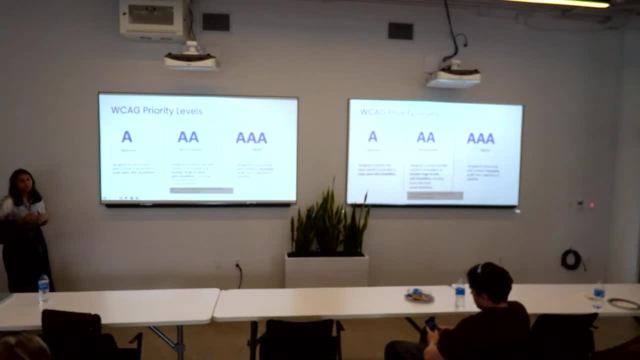 We need to know that the results of the test have been discussed. we need to develop and we should go to the next round of the test according to the current information. The third one is the quality level of the test. How to achieve the quality level of the test? 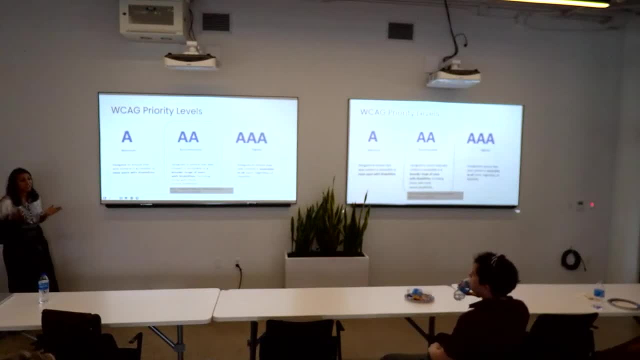 There are many companies that are failing because they can't understand the quality level of the test. So how to achieve the quality level of the test? For the quality level of the test, we should use this method Because for us to achieve the quality level of the test, 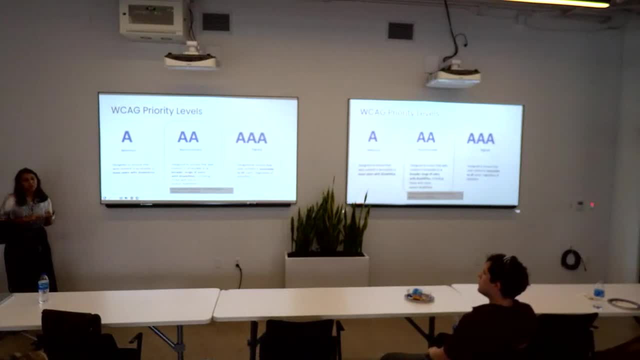 we need to provide the quality level of the test and we need to provide the sign language of the translator, Because we want to make that clear with the sign language of the quality level of the test. The other thing is that we have a website that we have seen in the United States. 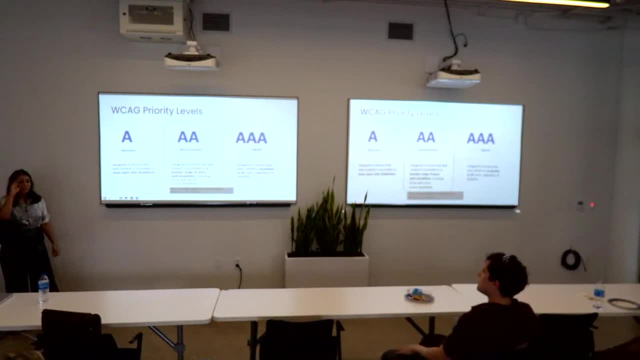 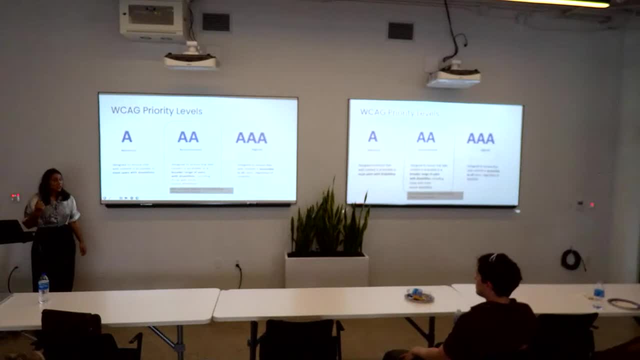 We can't have one second. therefore, we have seen that we have to figure out how to do that. So we have to make sure that we are getting the data, to make sure that there are flashing pictures that we can upload there. There are many web sites that they have to sign in the web. 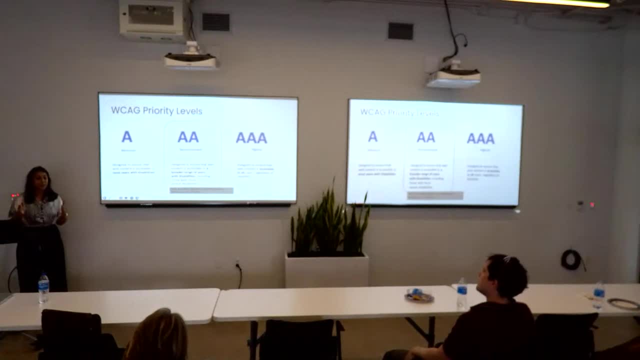 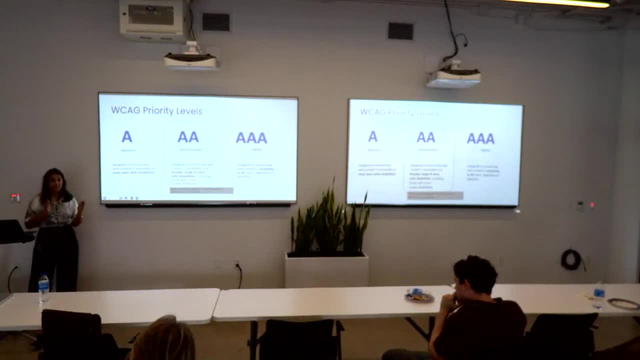 If you have a website that has these types of, you know, people with diabetes, you also have to do the testing that you need to do the testing to extend the time or to postpone the time. So that's how we can make the order. 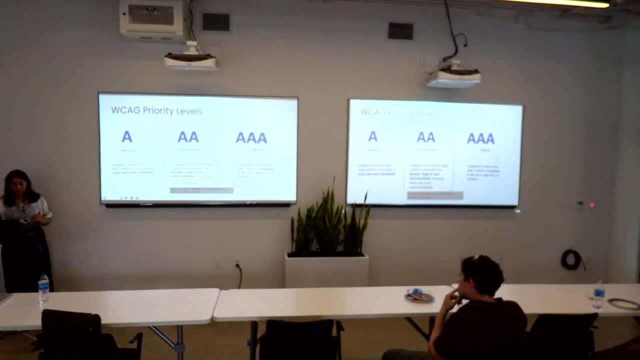 and make sure that people can use the information that they need to do the testing. What are the common mistakes we would put on the website? So, as I said, we see incorrect again if you can't put in the data most of the lifetime. 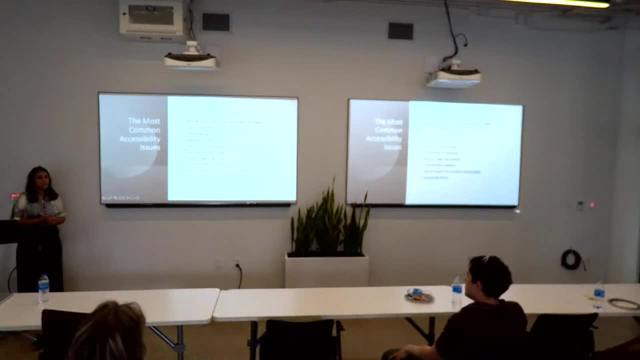 we want to make it proper to our alternative and if we can't put in the data, we don't want to use the data. It's hard to have that Low contrast, Low, low, low contrast. So there is no proper contrast. 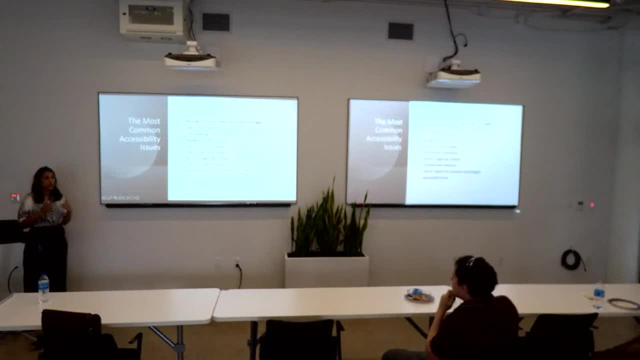 between the code and the actual data. We also have this problem that we have to use the text for more time in order to make the text to be visible and available to the user and the user. So if you, if you are using the text, 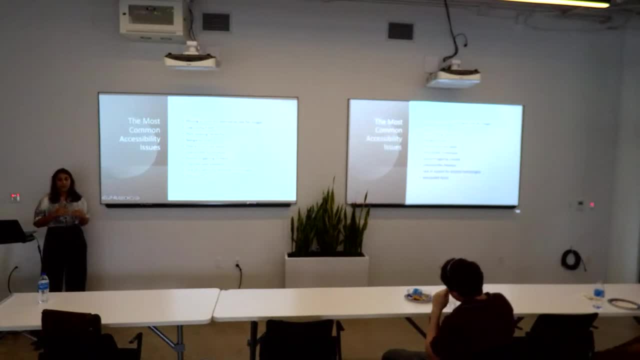 for more time. for example, you were using the text for a long period and you're using the text for such long period and you want a little bit to mix the other text over the text. you want a little bit to mix the text. 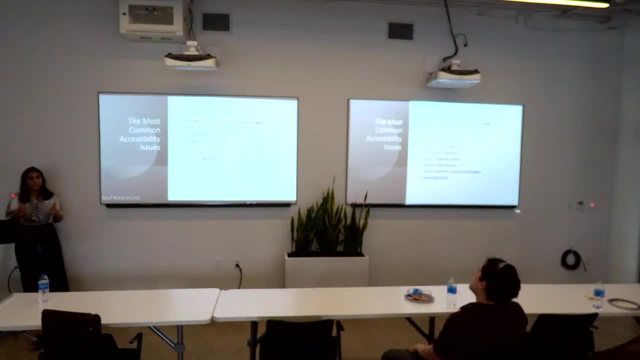 over the text. Why many times teachers make it so much? because they have many terms which are not using that text for a text. for many times they use the XML, The navigation. as I said, you should go by the proper name for the navigation. it is. 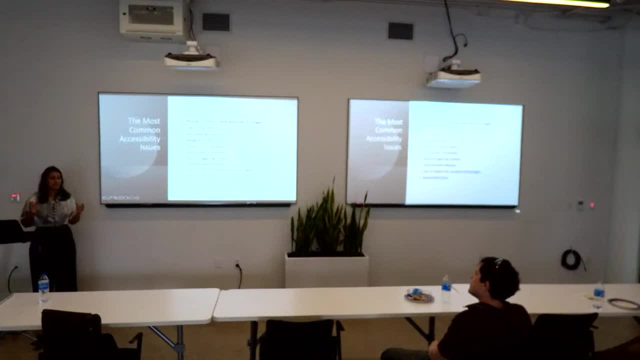 not just say that it is here, Or, if it is, just go by the name that you want it is here. You don't want to get the idea of what the purpose of the navigation is, so you should go by the name proper, like purchase, checkout, proper navigation. 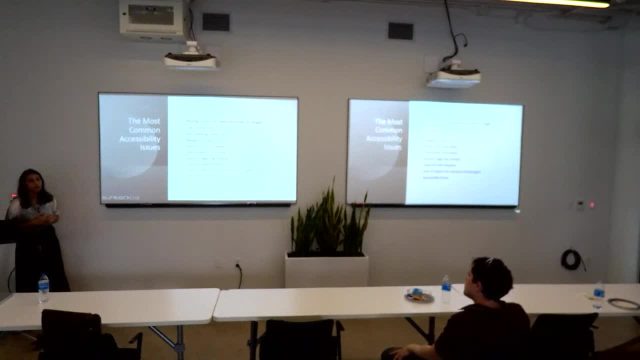 One is structure label. so if you have an issue with the first name, last name, password and so on, password, you should provide the proper name first and last and not just say go by the label for the navigation. If you don't know what is the purpose of this, then you should go by the appropriate information. 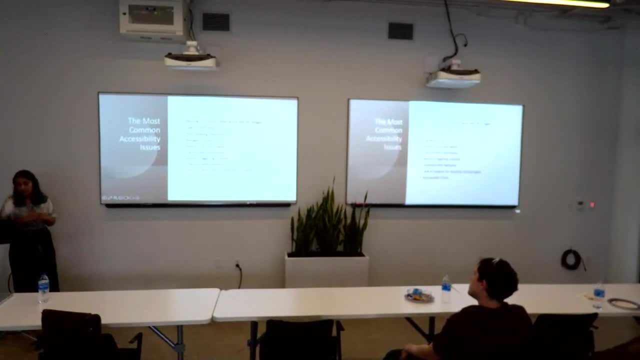 in the input field, Meaning, if you don't know what is the purpose of the navigation, then you should go by the right information and type it by the label. Now the students go to school or university class, so then again the Bo�ル would convince. 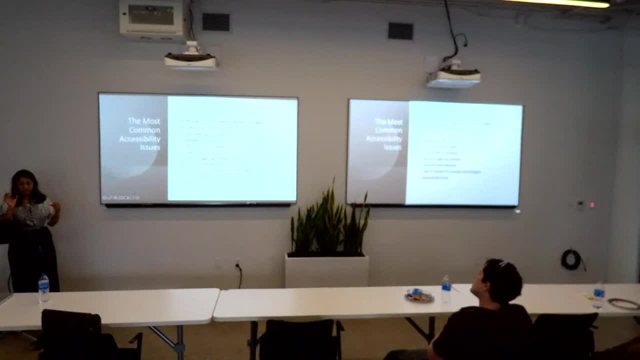 those students to go by the. Whatever is the purpose of this? and it is not just to say you can this and number You can do whatever you want. or here you cannot do that at all Because there are the. all the developers know what the HTML is, but they don't know. 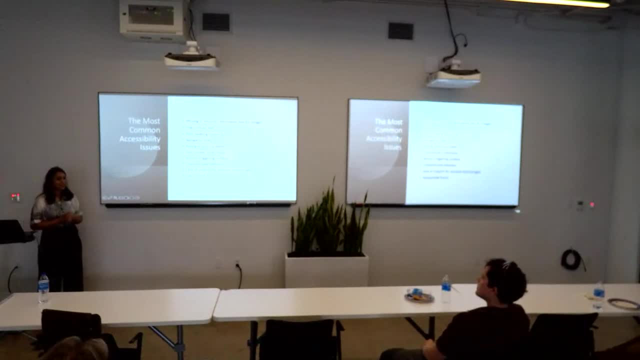 what the different is in the semantic and artistic expression. So in many cases HTML is an integral or artistic functional expression for the various artistic headers, then artistic methodology can be used to create these headers in the name of the header. You can use it in any case any application that is not an HTML or HTML, but it can help. 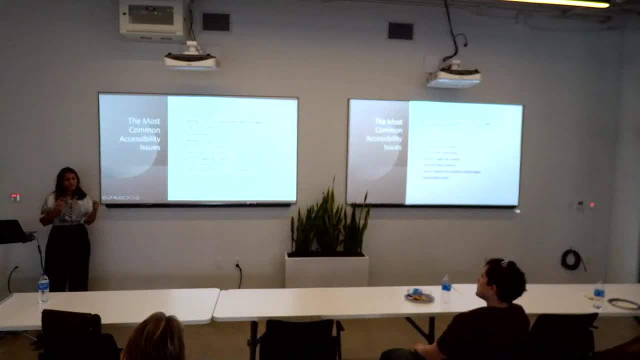 in the navigation, But in HTML. it's not an HTML expression, but it's a bit of a path for the customer to use And we think of a step by step path. then you have to go and refer on the level of this. 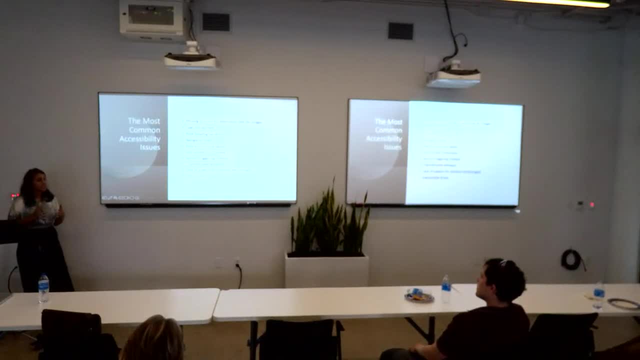 as properly. you have to look at the application and look at the application. It is a similar type of application to HTML, but it is a little bit more accurate than your humbler application. then you have to look at the work you do and look at the work. 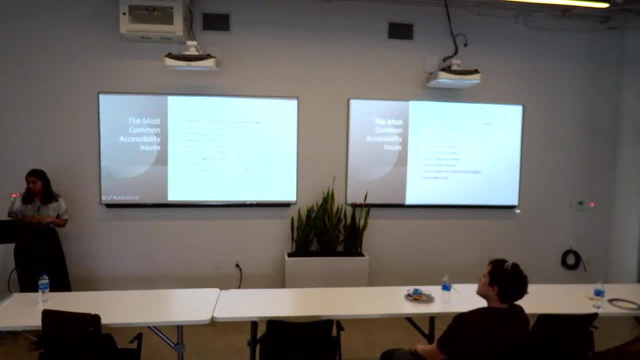 you do from the answer In a particular conference. we have a form. it doesn't have to be proper header message, error message that doesn't have a proper label and doesn't use the proper button name. so that's why I think that if you are familiar with the 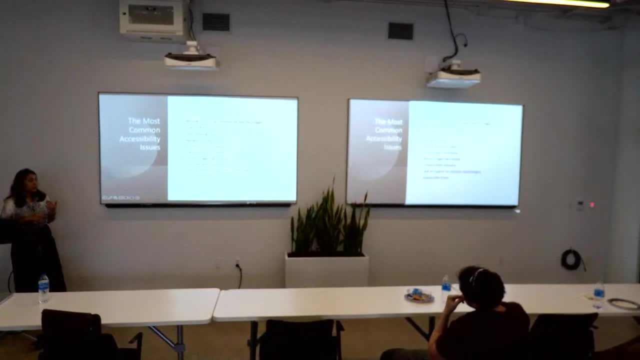 facial recognition of forms. you might be able to use that form with a proper error message, proper button name. in the last part of the video I'll show you the preview. so usually there will be one more opportunity to check the form one more time. 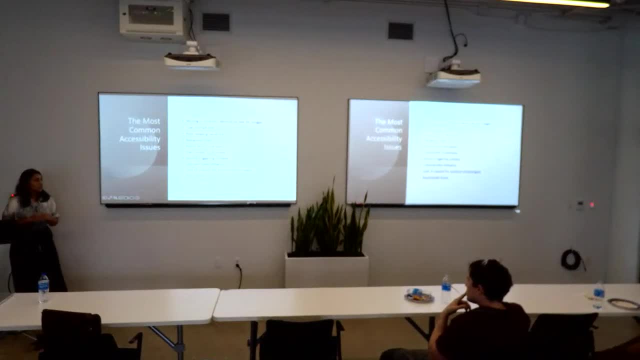 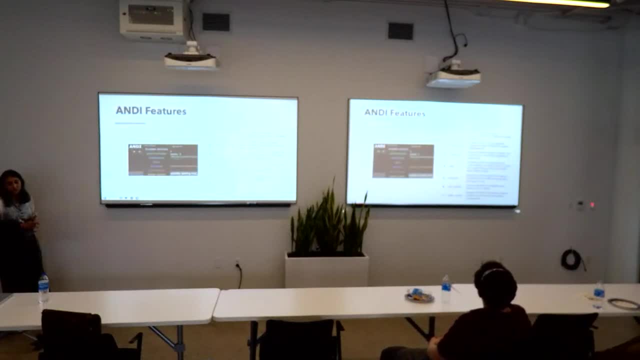 This is how it will look like Today. we can check if the element is protected or not. If it is a lacquer paint, we can check if there are any defects or not. If there is water on it, we can take a look at it. 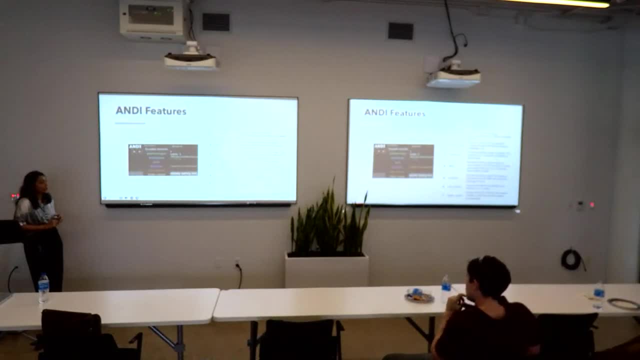 If it is overlaid, if there are labels on it, we can check. We can check if there are proper use of HTML or HTML. We can check whether there are some errors or check if the attributes are correct. There are many issues. 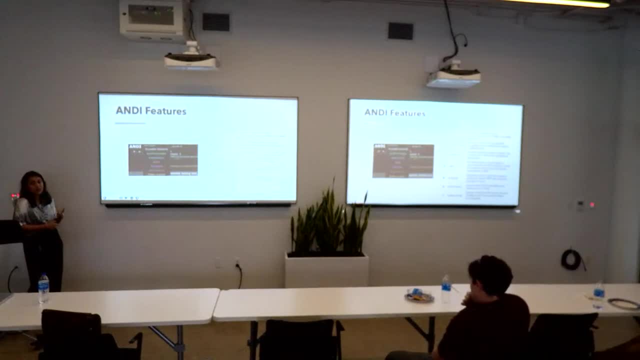 We can ask if there are any device. we can ask if there are any difficulties with the wrong password, For the password it is very, very difficult to get down, So when we do it we can ask if it is good. 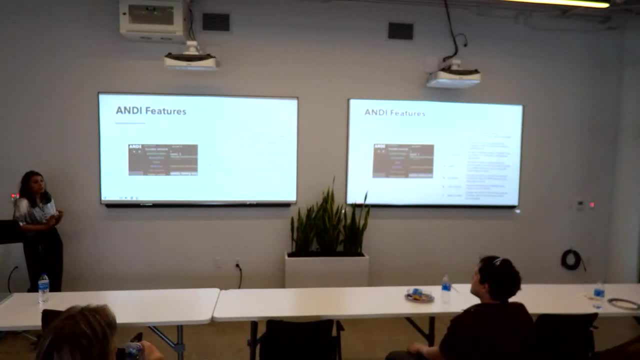 But when we do it again, we will run the software. But when we do it again, we will run the software And we can also check if it is correct or not. So this is what we can do. So we can check if the code is correct or not. 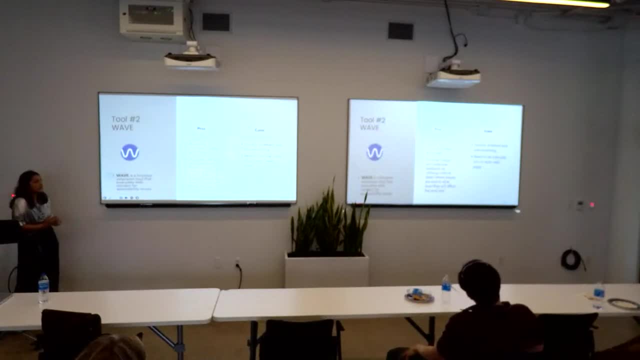 This is also a browser extension where you can go and view the URL and if you want to be a manager or if you have a current position, you will see that the browser is correct. If you click there, it will show you the URL. 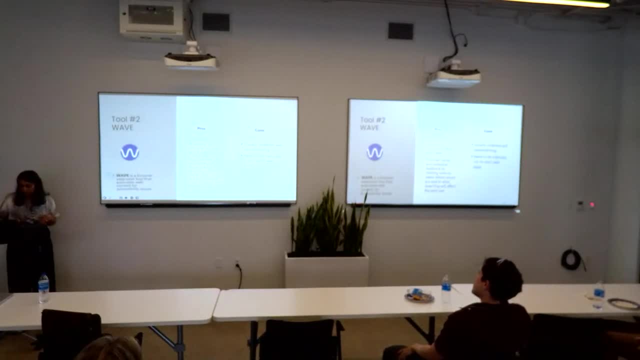 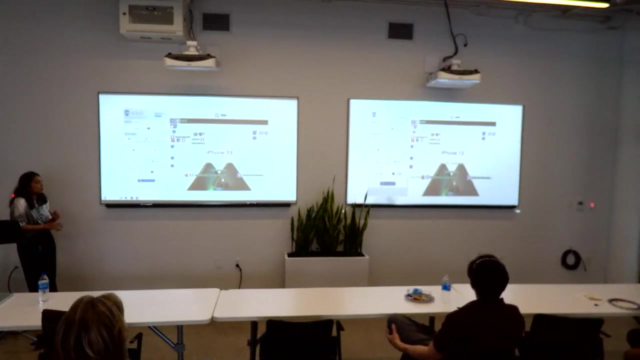 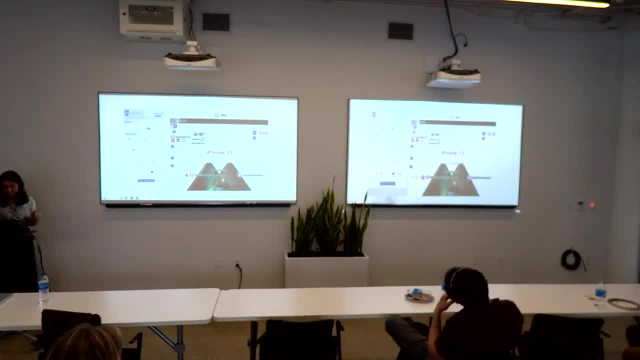 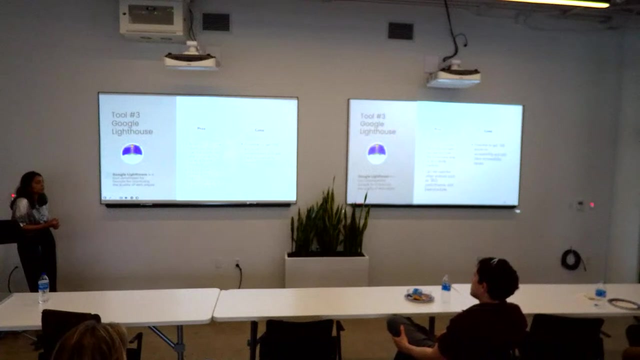 catches that error. Otherwise it is an error Alright. So right, we have done it. So I found a lot, of, a lot of a lot of people that are in the interview and the flow are in the flow, but there are a lot of people that are in the flow. but there are a lot of people that are in the flow, but there are a lot of people that are in the flow. 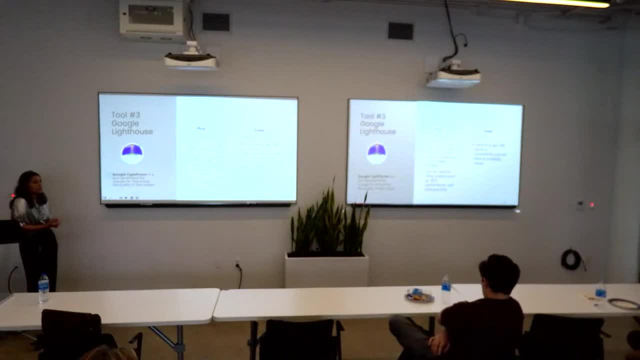 So I found a lot of people that are in the flow, but there are a lot of people that are in the flow. So I found a lot of people that are in the flow, but there are a lot of people that are in the flow. 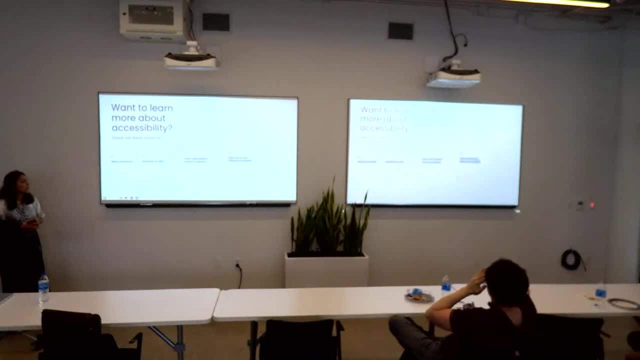 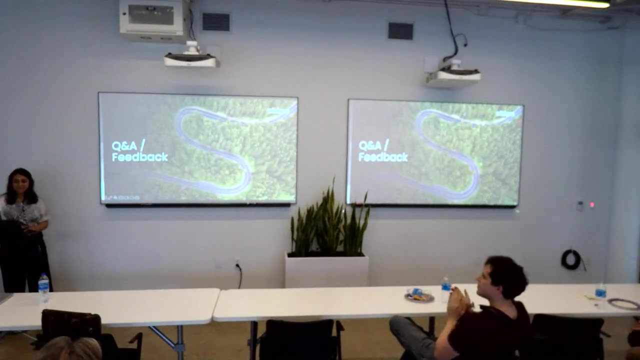 So I found a lot of people that are in the flow, but there are a lot of people that are in the flow. but there are a lot of people that are in the flow. So I found a lot of people that are in the flow, but there are a lot of people that are in the flow. 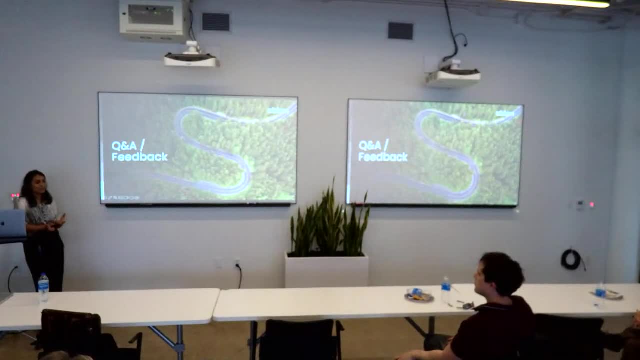 So I found a lot of people that are in the flow, but there are a lot of people that are in the flow, but there are a lot of people that are in the flow. So I found a lot of people that are in the flow, but there are a lot of people that are in the flow, but there are a lot of people that are in the flow. 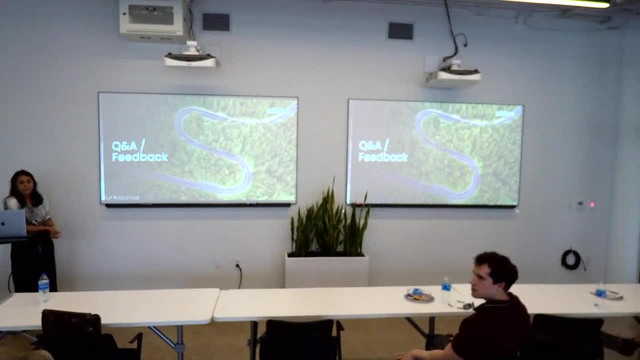 So on the automation side, you said it's difficult sometimes to do the automation. Can you elaborate a little bit more on what are the challenges and part of making these possibilities? So, as an example, if you are in a city like town, there are some communities that have 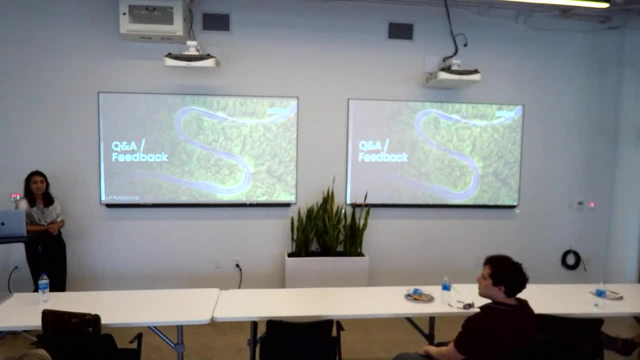 a lot of places where education is needed. for them to be able to do it, They need high-tech buildings, And if you are in a city like London, there's a lot of issues where there isn't enough education. So I want to share my experience. 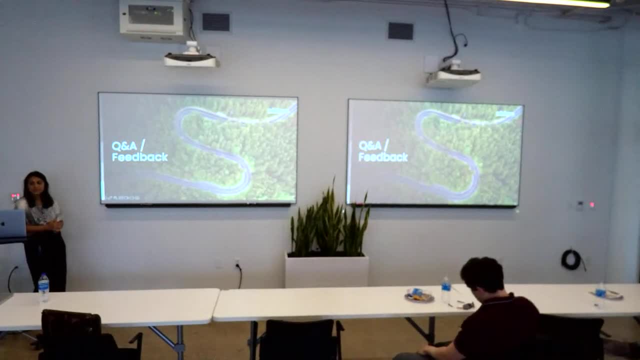 So like we integrated with Xcode? Yeah, So it's open source library available, widely used by maybe all other tools as well, But there is no guarantee that we can do it. But yeah, it helps to identify 70%- 80% of those accessibility issues and point it out. 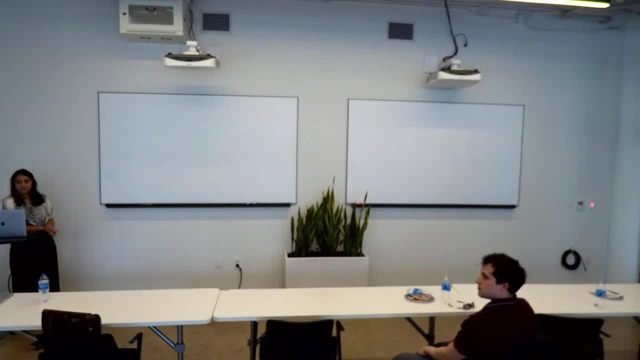 in the right direction, Like: what is it? What is the issue? What in the HTML4? you need to fix it, But you cannot be very, very confident all the time. 100%, I mean it is not covering all the aspects of the accessibility system. 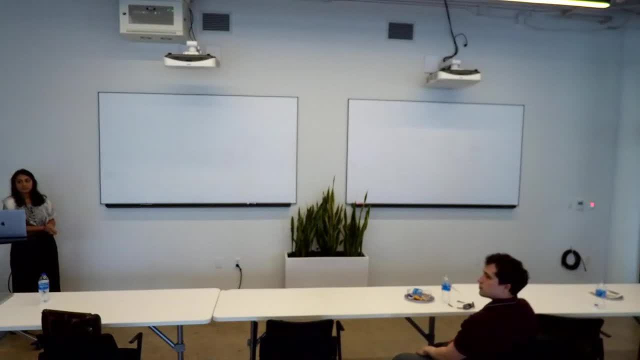 So it is about one of those things. But like they have, like it's, they have through and they can, they can go to the next step by just clicking the. But there is another challenge: is the flaking, like that visual stuff that they can do? 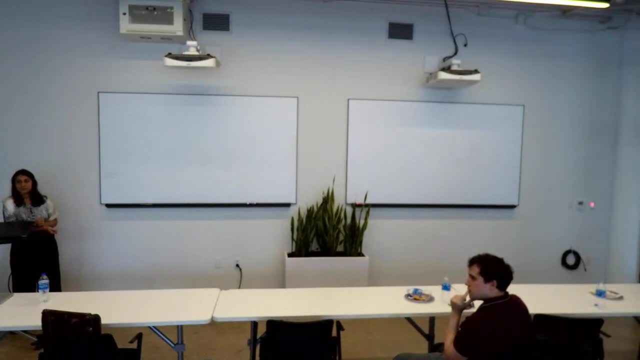 You know the visual stuff that she mentioned, like what flashing in like three times in one minute. It is not something more like you can get it by a. That's more of It's not. It's not so much that it. 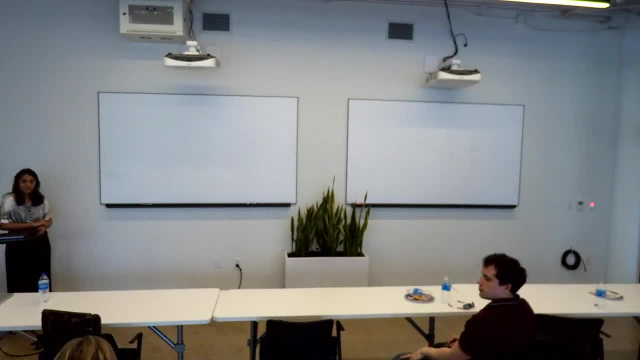 I'm sorry to interrupt. Yeah, Yeah, So I was just saying that. no indication that I get that. Yeah, What about the AI? is there any role for AI in the? so one challenge obviously is the common denominator right if you want to make that web experience that maximizes all. 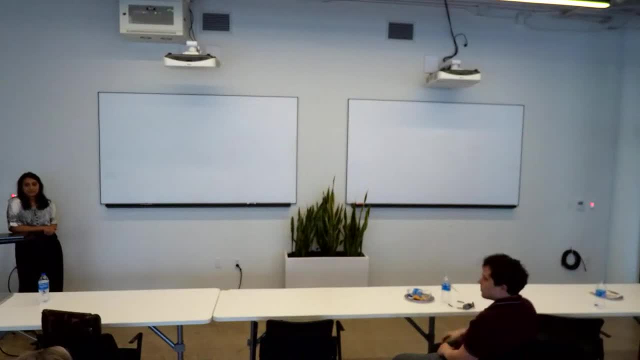 your senses, normally like for everyone else. so it's a concept of adaption. but you know you have pages that sometimes can change depending on the size of the screen. right, so that concept exists within accessibility so you can identify as clear as might, and then you 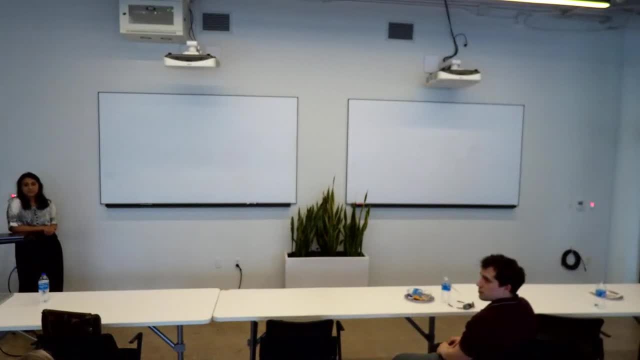 can render it based on the knowledge it has and put AI in to help you re-render it. so I'm just trying to understand some of the state-of-the-art in accessibility. I'm not sure it's me, but let me just answer because I wasn't thinking about it, because 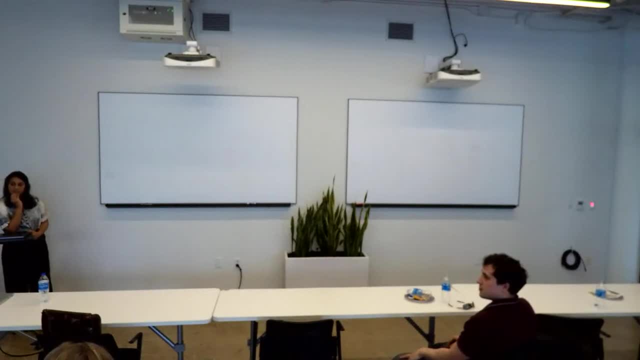 what I found was accessibility is based on the rules, right the rules, and it also has examples, so it is a very good scenario to train LLMs with this kind of knowledge right so it is not outside of the box, it is not something like a random stuff. it is consistent, right and 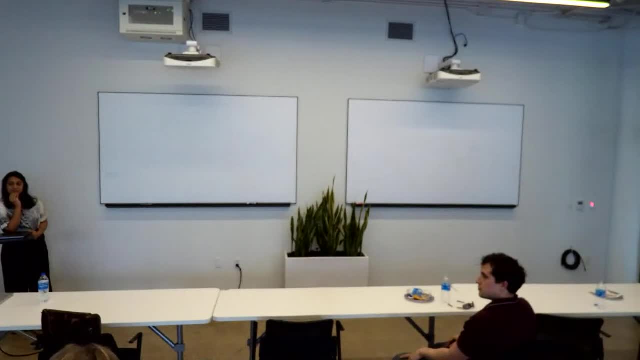 now we have an open AI for all the LLMs out there, but also, like you know, for example, like a Gemini kind of LLMs, which also scans the video, right. so I think, yeah, I think this is a perfect use case. yeah, it is up to the like. who tells us? because I was. 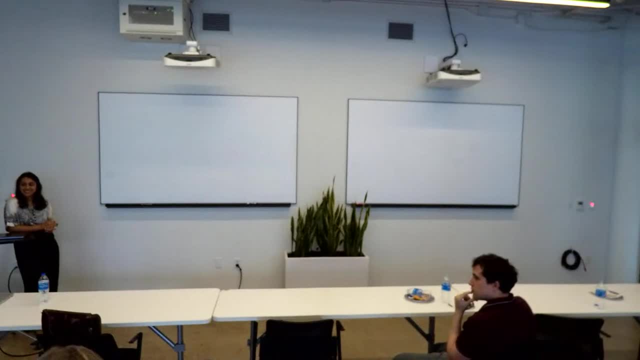 when I was talking to her, because we are doing like X level of stuff. but if you want to be precise and be confident, then, yes, technology is there, it is getting better, it is getting better and better and better because, through the video analysis, through, 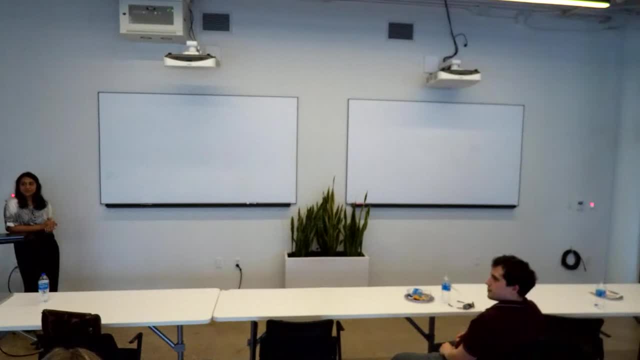 the image analysis you can say that it is able to do it or not. so we have automation. so to take care of the like medications can be done- by the tabs or not, is the medication doable or not? but also wherever the automation cannot do, where does this Gen AI can help? 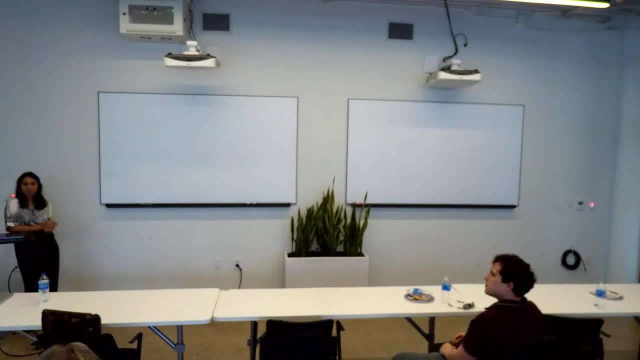 us out, yeah, And also there seems to be a dependency on screen readers, right? You know screen readers and their secondary tools that are external to the application, right? So, but that's a great challenge, right? Because then they have a third party tool that kind of looks at them and tries to do. 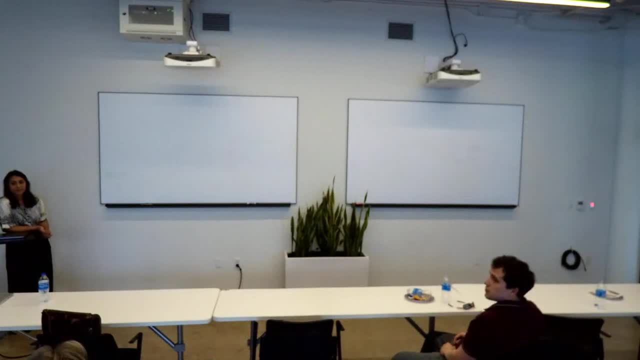 that Is there. you know, standards, objects where you can, like I said, where you can kind of create a profile, like, for example, the browser now has a simple page right When you remove some of the lines, you can just read more easily. so is there something? 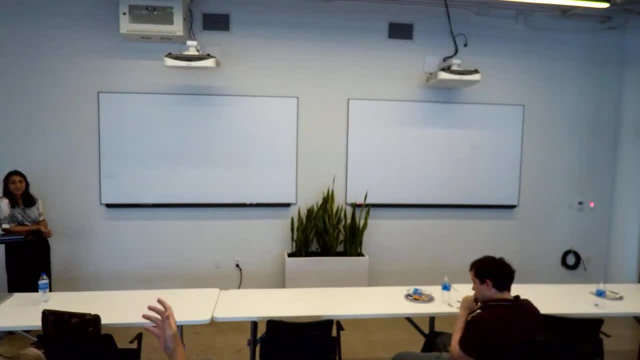 that you can identify. Yeah, I'm not sure that's the key or something to that, to make you want to render to your specific disability or disability right instead of being, instead of trying to minimize the page so that it works for everything. the problem with that is like the least. 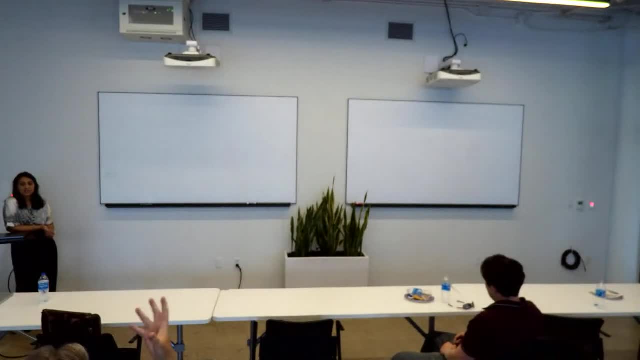 common denominator, right Yeah? Like, if you can't have a flashing color, well now someone who could benefit from those doesn't get to see them, Mm-hm. So you want some sort of adaptive, or I'm just curious? 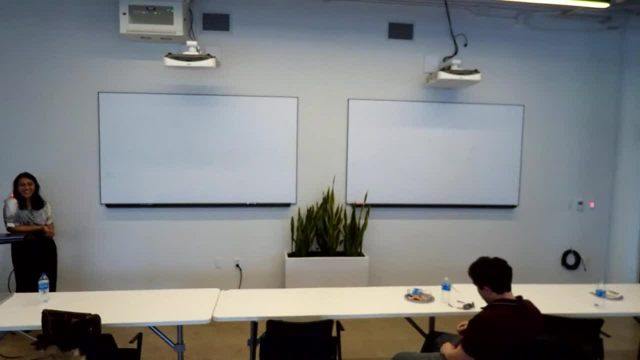 I know a lot about accessibility, but I just think it's an area. Now the problem obviously, like in everything, is it hasn't always had a focus, because you know market share and I know you've heard the numbers. but I think with the laws becoming more strict, right and there being consequences, you know, I could see this being an important area. 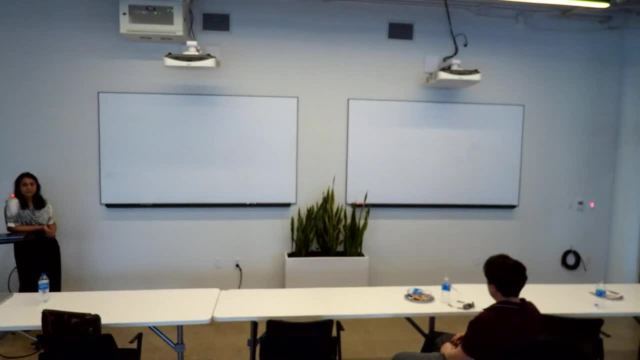 Especially also in the application, where you already have a lot of webpages. you know how do you test those that you can't, So this is a part of how you can reference it. Yeah, so what I learned from this, you know, is it is not only about pagers or demo, but now the marketing, like it is about graphic design, because they also need to be adapted. 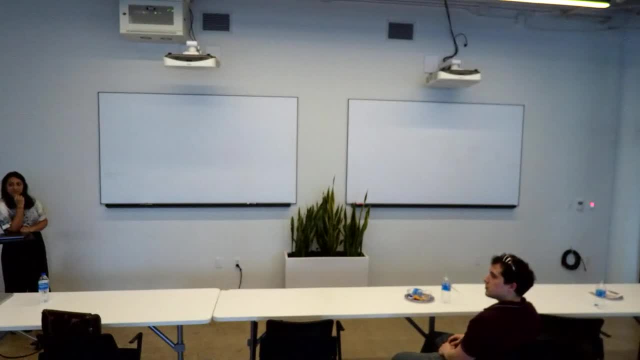 They need to be the same. Yeah, So most of the time we put what they provide us that hey can you put on this website and we do it and we don't know it. Also, the product designers needs to think of it like the path and also like 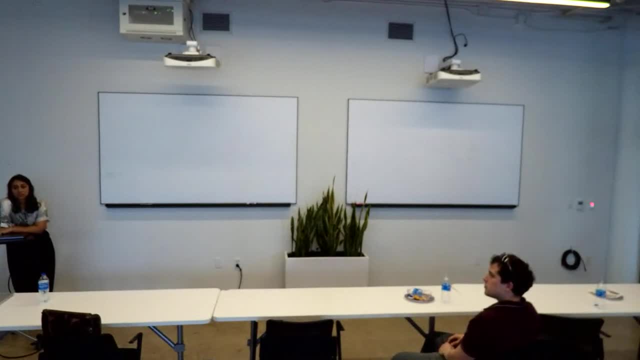 They. they are going to have to keep up with the experience, Right, Yeah, Yeah, It starts from the data department, Right? So that would be greenfield, right? So if you know the Yeah, Yeah Meaning from your head, though, that would be easy, right? 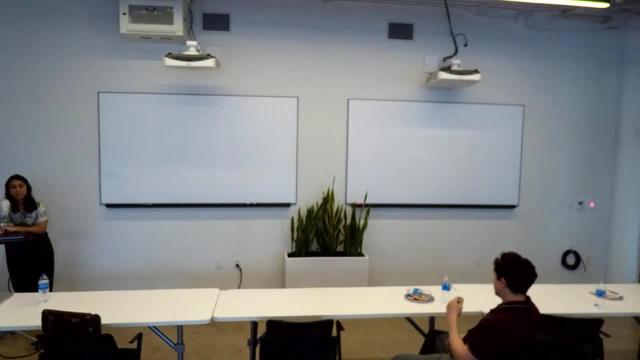 Yeah, So the majority of the stuff is already out. So if you have a retrofit aspect, it would be helpful. I think this is something unique. Yeah, use case that browsers would have by the people that you mentioned. right That based on the person idea or based on the? 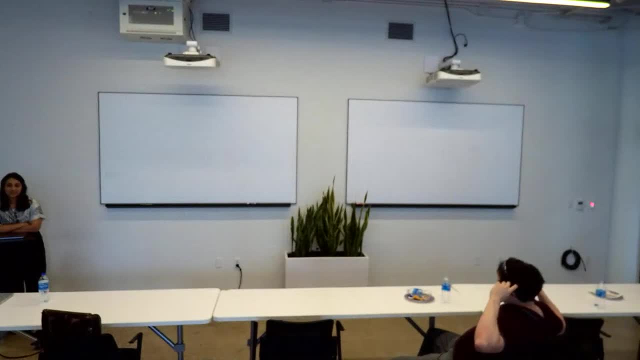 Yeah, And the profile. as we just said, I have color one And so now the browser automatically write every kind of code that would support rendering the profile, to support rendering the color blind burden. but I don't want to see color blind. I like colors. I want to see color blind because I don't want to. 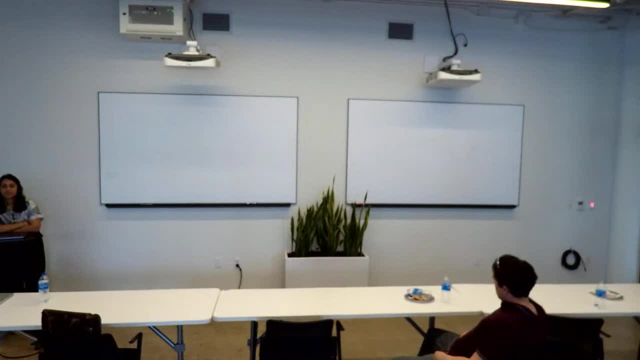 so it's a hard problem we could be trying to solve. I think it could be, because I know that yes. so then you, as the conference provider, lose control of that experience. so that's the external problem. if I go and I let's say I have four sides and I make the formula large, 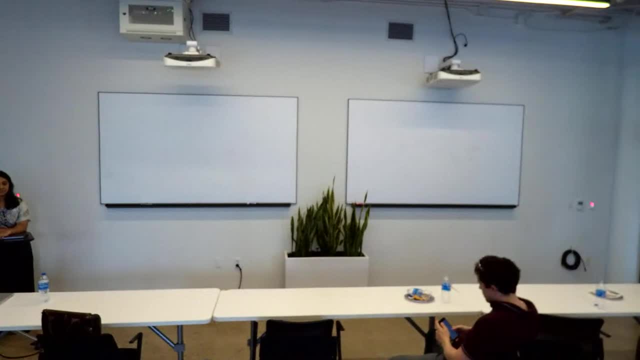 all of a sudden you find that. so that's that progressive behavior. that's very important anyway. so I'm just asking. I'm not very much in this field so far, just curious. no very much, so I'm not sure if you have a knowledge of. but there is another question came to me. 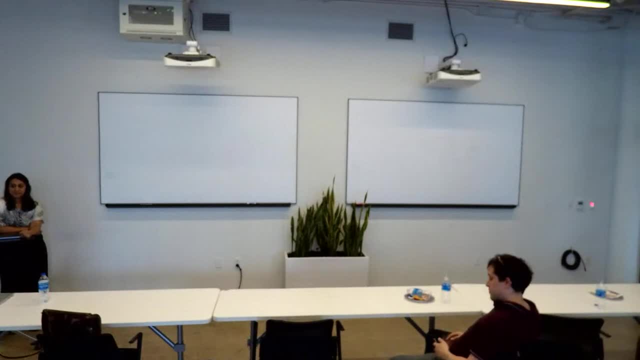 like I have some simple food website. my users are very notable to me in PCC in the very small budget shop and I don't know, like, with these regulations coming down in future, do I need to be accessible because other people might not be my target area? 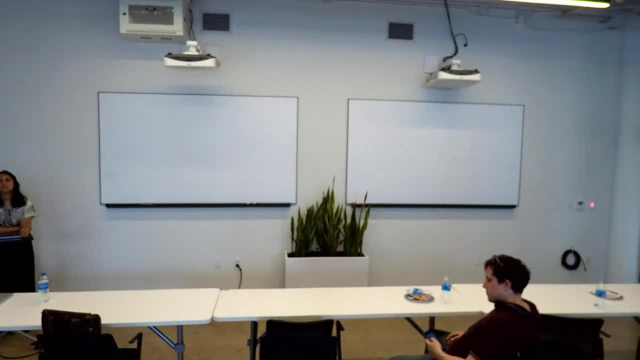 or what. that is not something I- I cannot use the word- care about it, but that is not my focus area and I do not have the budget also to have that kind of very custom people website to make sure to hire those accessible experts to review that website. 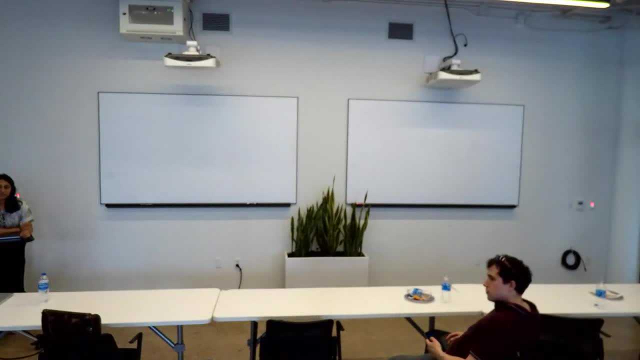 it might be that just wordpress or wixcom, I put bunch of images to the website, so I think this kind of brings the red tape on the businesses or those who wants to operate on the global budget, and that's why tools and platforms help. because if you could say 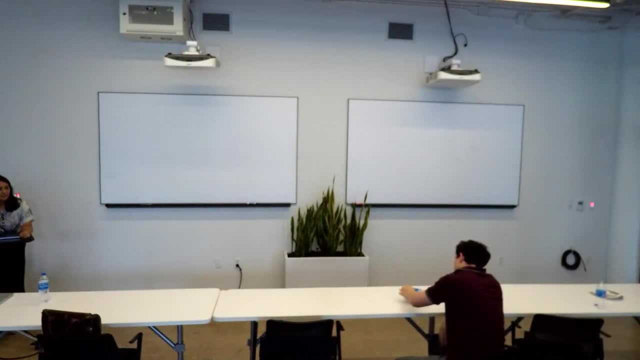 when you do a video, there is an AI module that automatically has the option to turn on. I might you can go turn it on. so now I, as the user, can be paying for that if I want to pay myself. that is not the content provided, but it just has to be simple. 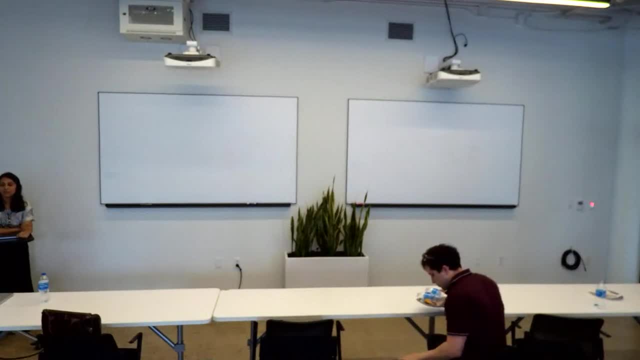 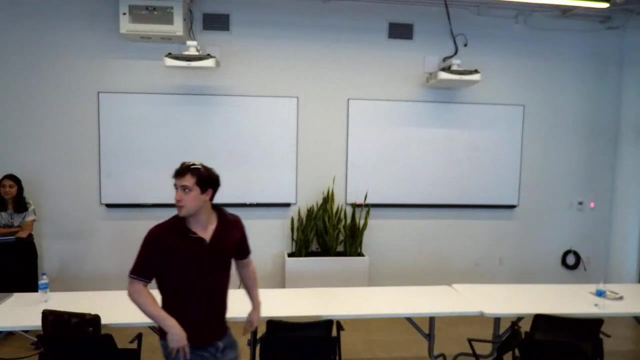 and easy. this is an interesting question, but I think it's a similar issue to average. when you have different insights, right, they have to come up with a solution. I want my page desktop, but I want it to render on a small device, on i9. so do we have to do? 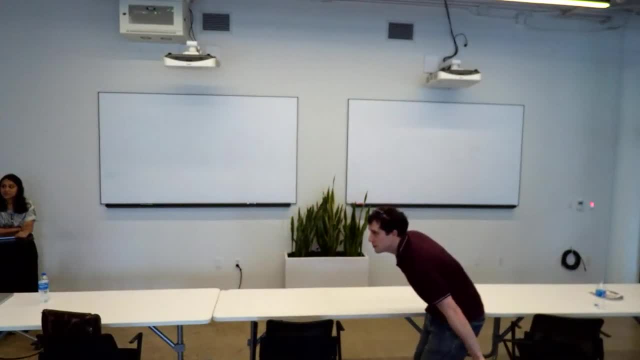 progressive pages. I haven't seen them all. how's it going five years from now? probably that's COVID, pre-COVID. why is there no organizer for this? there was no organizer management before the registration. oh is there? I was like, yeah, we put an event right on. 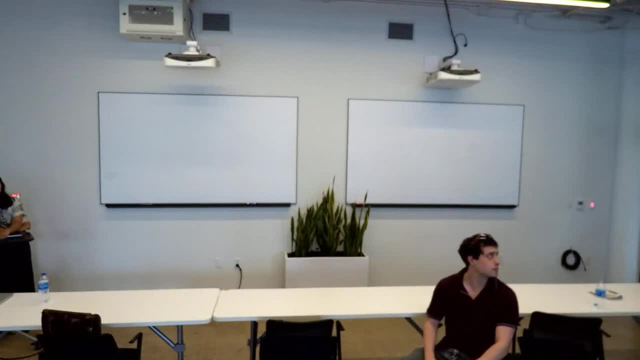 but this is my first event so please excuse me for this. I attended many of these capital projects, but this is the first time I'm hosting, so I'm loving the process. normally when I'm writing shows I could organize it. it literally was empty, I think, in the app. 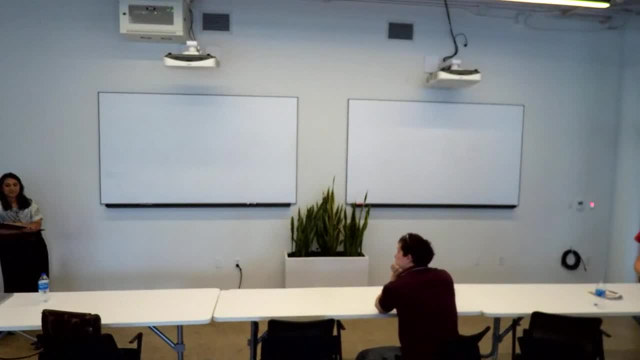 it actually says now that we organize this, so there's also no location. oh yeah, I pointed out, but I couldn't connect, so I asked them to do the live stream. so they have to do the live stream. but yeah, it's a good job, I really appreciate it. 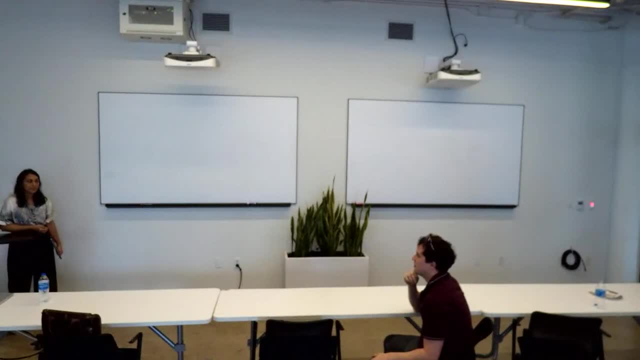 but any VR experience other than this, what's the experience for you? you don't have experience with it- very little. for my last job, we were starting to do it before I left, but we were talking about doing it for the current world, so it's been very supportive. 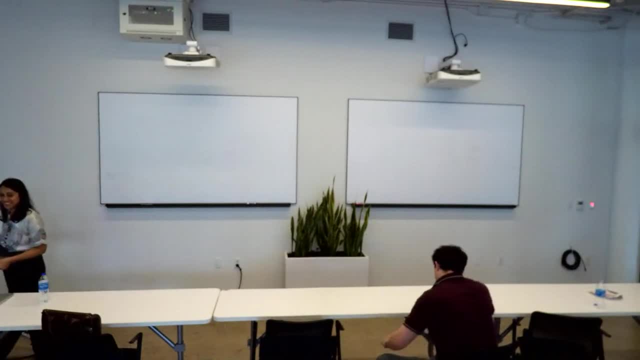 thank you, thank you very much for everything. thank you very much so. yeah, so I think this was my first vertical scoop that we showed up, so we'll not have much more, but what I want you to say is: yeah, please share your thoughts, like what would be. 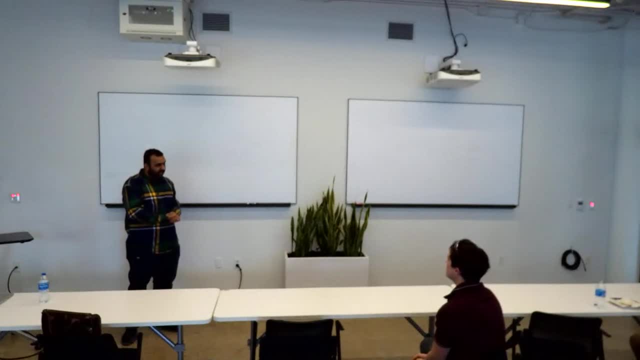 the next topic. if you would like to be present here for the next testing related topic, I would be. I think our next will be on the first of May at the same location, and I'm planning to organize every month in the first week of the month. yeah, 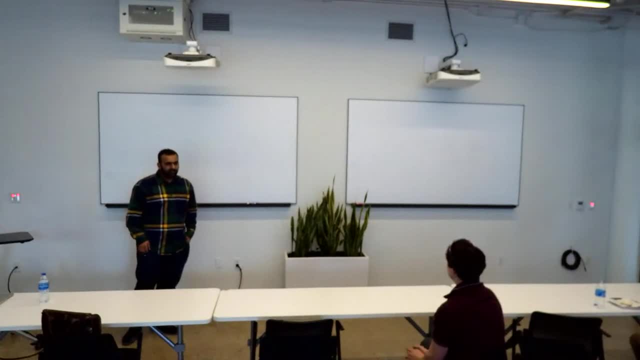 and on all the Wednesdays. so yeah, thank you very much for joining us. it's like you said: software can be set up in the library or the web. yes, so okay. so yeah, thanks for being here. so I'm coming from the software development and DevOps. 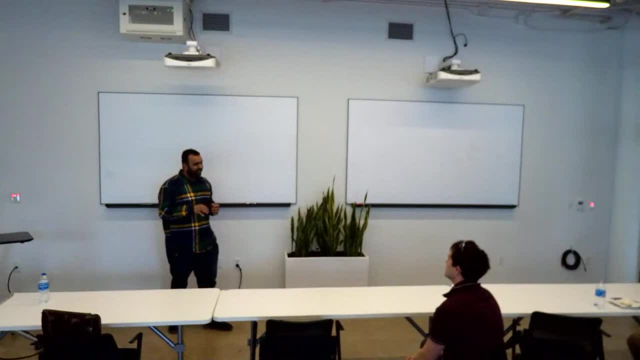 background, what I have seen is every day the push is towards the development of the software and the release function and, till now, the practices by the QA teachers. for a reason is still the manual software testing process- and manual doesn't mean that, but still it's still. 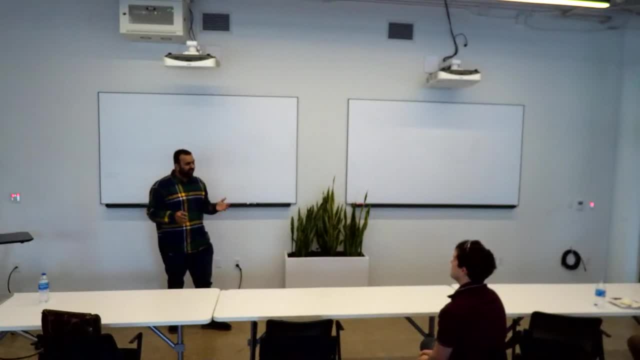 in the process. okay, and now QAs are very limited. like we have four people out there, there is only one QA or ten team members, two to three, and they also need to be struggling with delaying the process of the release and also it is not possible as product grows. 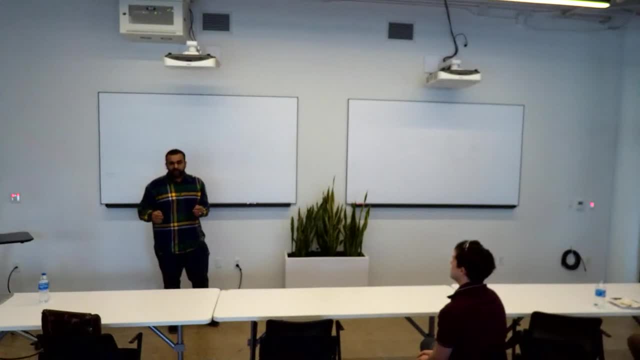 that they will be able to teach all the functionalities all the time. so they need to only touch the very important point, like smoke taste, and then after two to three they might need integration and all. but what it creates is issues in the product because they haven't. 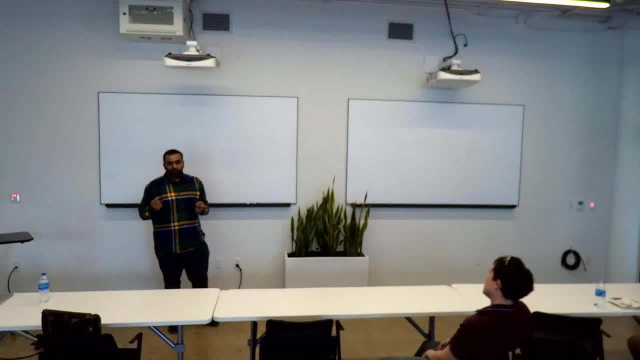 tested everything and then the value of the QAs are not correctly visible by the leadership teams in all the order. so what we are trying to push QAs towards, what you are doing, is very good manual testing, but you should come out of that just basic. you should be. 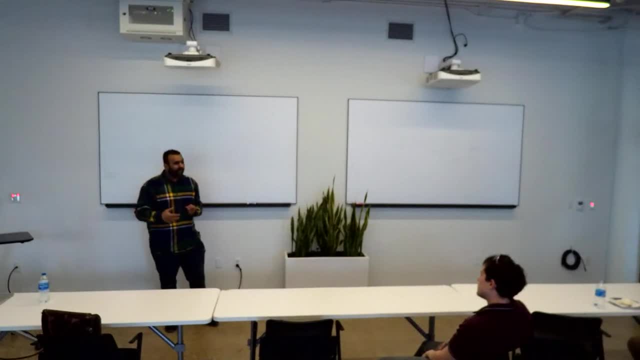 thinking about your products, performance. you should be products accessible and more. but how? without using tools, you will not like how and all these things. you need to come up and orchestrate yourself with the more tools around you so you get the time back and you can do. 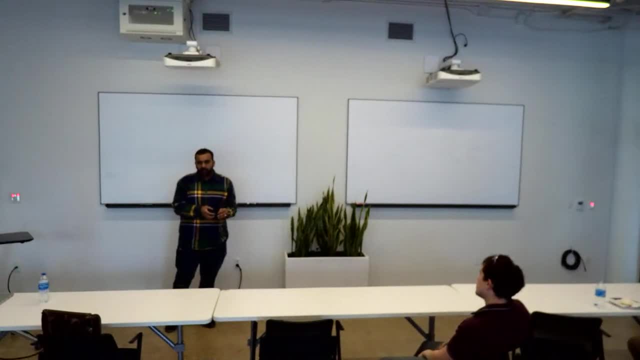 the four times of testing. so why DevOps? because the tester should be the co-pilot of the developer. so they shouldn't be only saying, hey, there is a bug, there is a bug. they should be saying: this is the bug, this is the evidence, this is the offer. 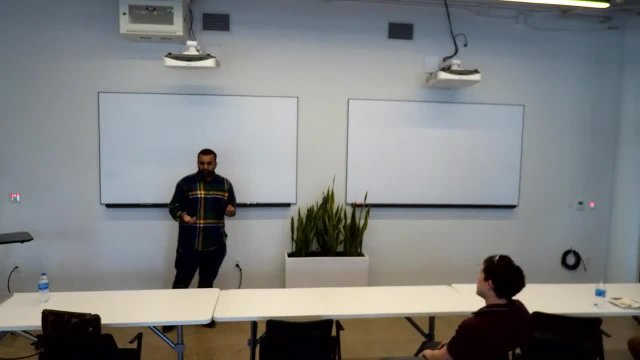 so this is the terminology that the tester needs to build it up. they cannot say anymore, say oh, it is a bug, it is a backend, so I don't know this is what data is using. I don't know. they need to understand the terminology. they need to understand. 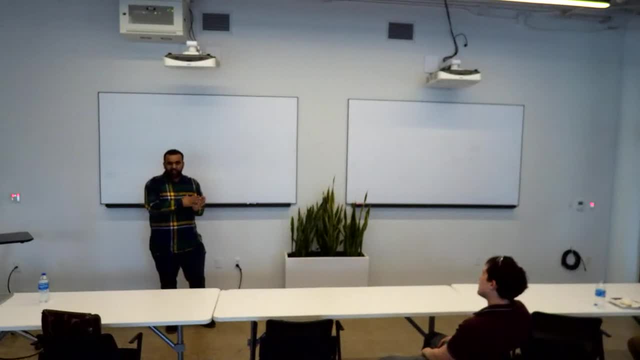 the context. so that's why, from the manual software testing, the transition should be the quality engineering and that's why they will be like 1% or 2% will be capable of finding using the different tools that we have in the same that we have. 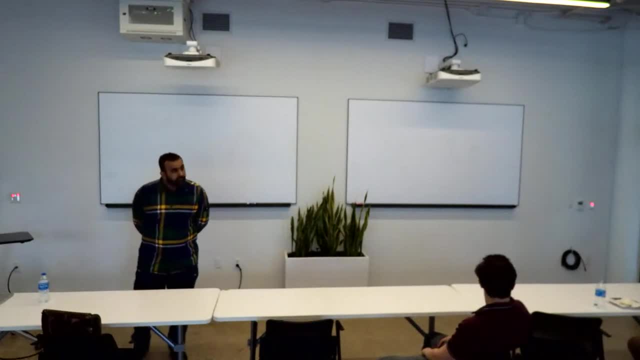 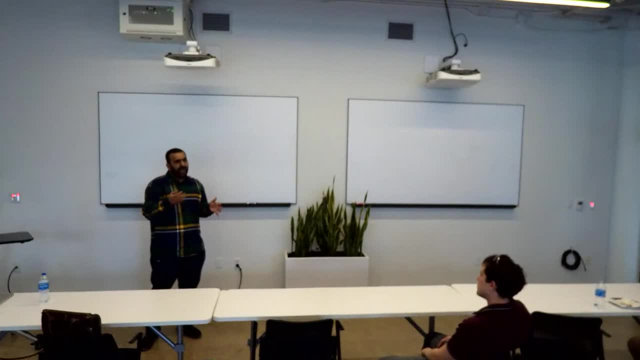 but practically achieving all the regular releases right and stealing the time demand right. you cannot stretch too much. so that is, we could say that that kind of started already many years ago, in the sense that first was software engineering and then UA got brought in and became the quality. 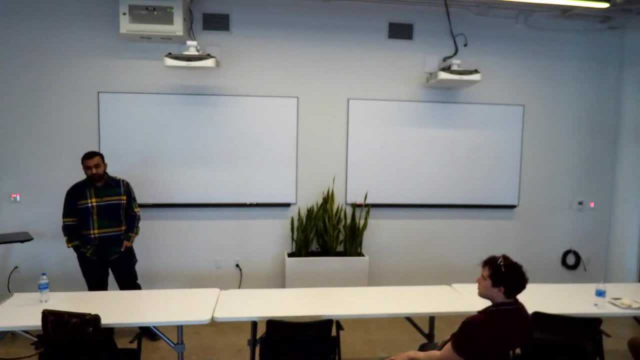 engineering, and now we want to build a platform that supports quality, and then that extended DevOps infrastructure, and then security, right, security. so this is the same path, basically. so you, you just is that what you are indicating by you know? so let me bring quality into this. 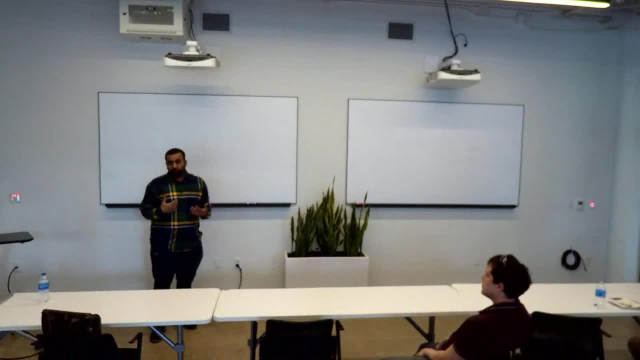 to the sort of practice or how. software, yeah, so like let's see one of the customers we are talking about on the wall they are. they have nine, three, four, five, six, seven, eight, ten, twenty, twenty, twenty, four, twenty, twenty, fifty, twenty, thirty, fifty, seventy, sixty, twenty thirty. 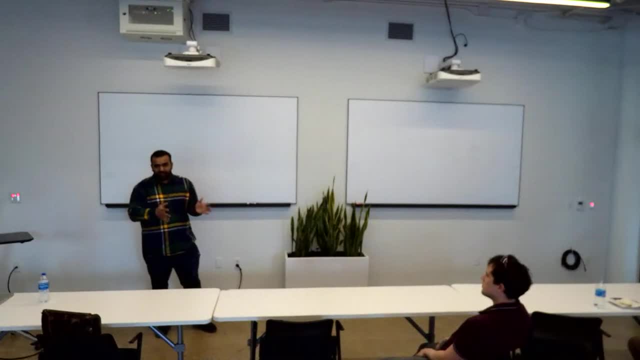 one, two, three, three, thirty, ninety, sixty, ninety, use the cadence and then do one week of development and one week of testing and or database, and then that and then release and making sure that the product is not broken. so they need for those patients to adopt the capability to do also right, so they need to automate. 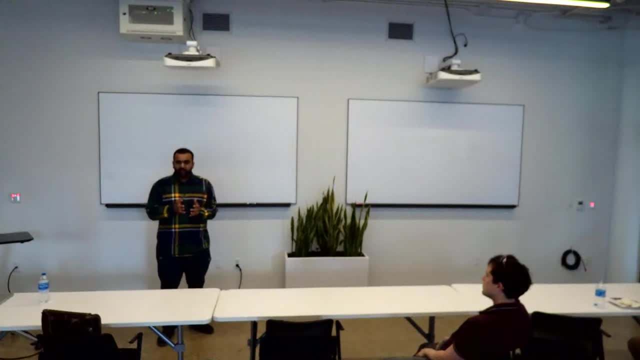 they need to do x, y and z. so that is one, but also that the, the information is being used by, like the idea of application as integration. they have apis, they have a big analytics pages where their manager sees the like, the sense, engagement, activities. so performance is also. 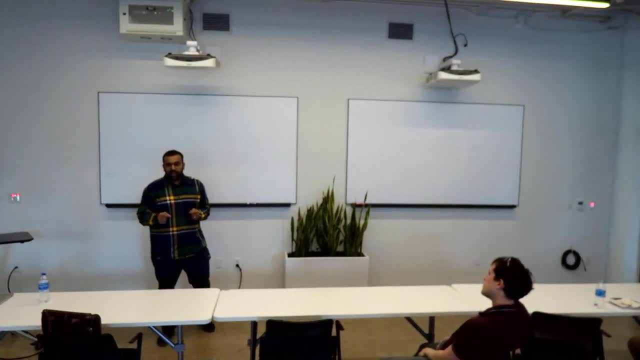 important aspects along with the functional based now it is, doesn't have the tooling in that place. so what they do is once in a while they run this live house phase and there is just just even point of that. it is not the consistently. they run like house for all of 600 bases or all the pages, because all page might have different data or 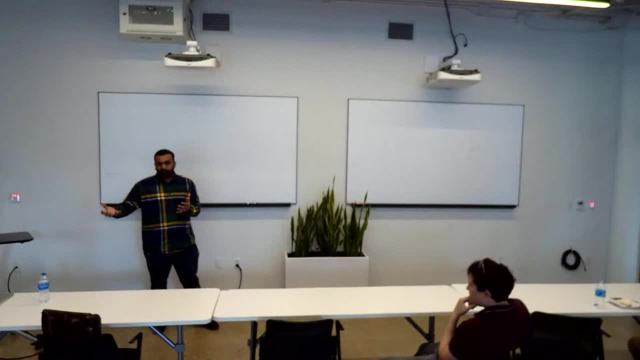 different data sets, so the at the time of their testing in a like, more traditional way, it doesn't provide the value that they're looking for, and when they base the similar application in the production environment, it's it's loading or crashing and each time out because it is more. 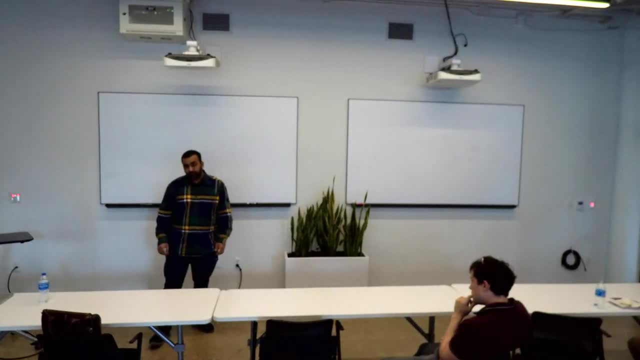 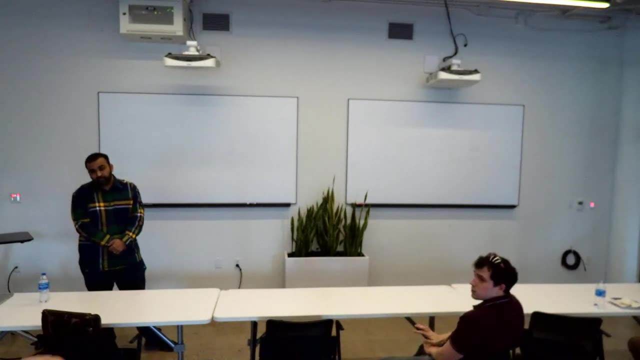 time. so, but you're describing that that's your only problem, because, ultimately, if you are, and then you have to, all right. so if you have ui tests, you don't want to do like that and there's also your reason. so that's, that's what i'm saying. 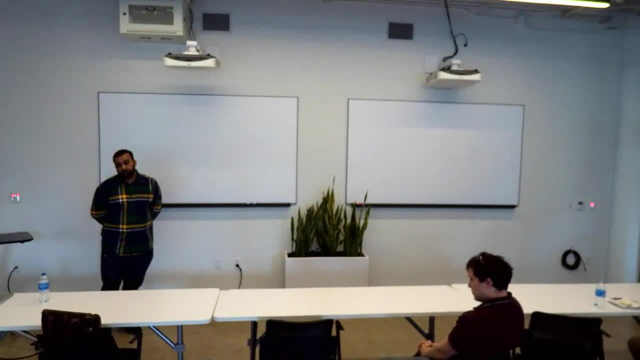 yeah, yeah, because when you mentioned about tables, so those things are there, but when it comes to the quality, or we need to increase the scope of those themes, because current srh only looks at the production. they don't look at, like, how it is being, they will tell you based on looking at the tools like simp3 and data. 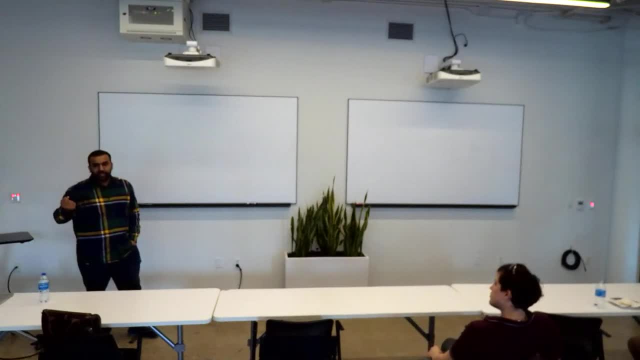 some metrics. they just tell you that, hey, this is the issue, but they are not taking ownership of the 451c now and they are not going to find it like it is very good, longer time and all those things, but they are not. there's some consistency during server incidents. 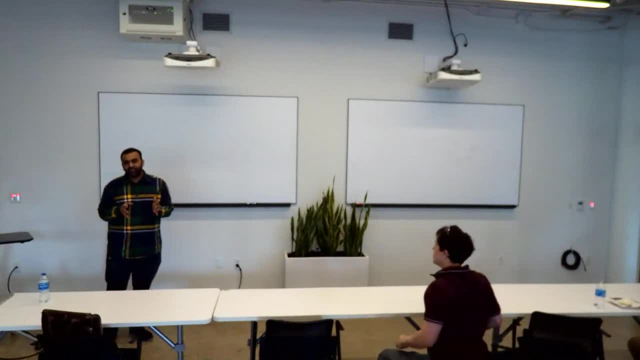 same for the DevOps. i was the DevOps but i was more interested in the csm during deployment: fast, fast, fast, but not taking care of the calling. So whenever there is a production issue, not of them, but all the patients were asking the same question. that, hey, why is? 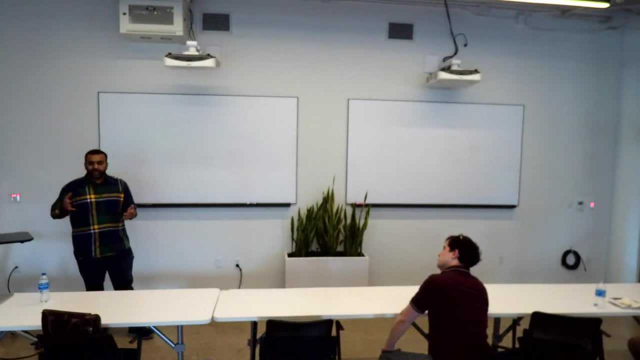 this issue in the production. We didn't do this, we didn't do that. So that is my point is: yes, there are things that might be the whole concept of quality engineering but, like QA is a very cliche that everyone says that quality is everyone's responsibility. 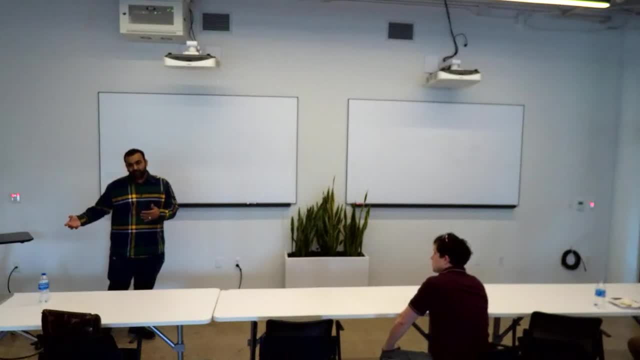 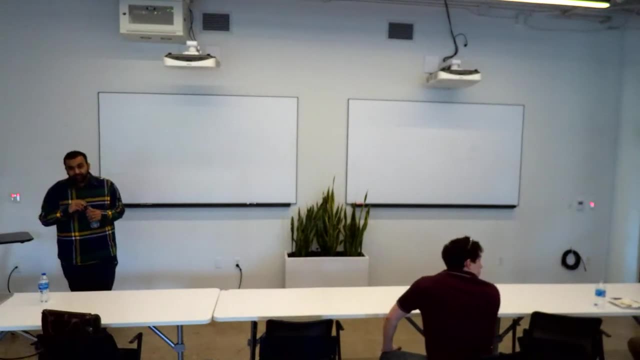 but ultimately those questions have been asked, And also because many times they are asking the QA team a quality control question, not a quality assurance question. They are asking: how could we deploy to production a product that has above, that is not like that, and 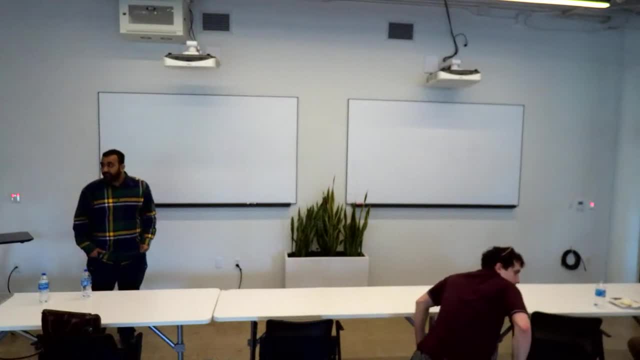 why should we miss it? But the communication that is going on is to bring that in. Alright, I just wanted to see if anyone needed a voucher for the garage downstairs. I didn't know we could. Is that new? because last time, which is several months ago. 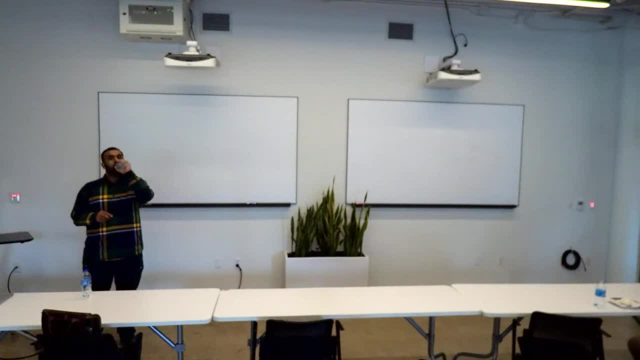 Yeah, if you come to a capital factory meetup, you can offer me- It's just a $8 flat rate parking Next time. Yeah, for sure, I don't need a parking downstairs at all. Okay, I think they've always validated for like $8. 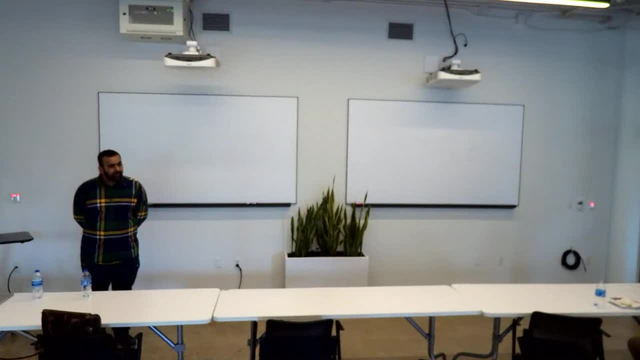 They do. I think you have to like, enter after 5 and exit before 10.. Maybe that was how it's zoned. Yeah, I think, like if you enter before 5, I don't think that validates, I don't think. 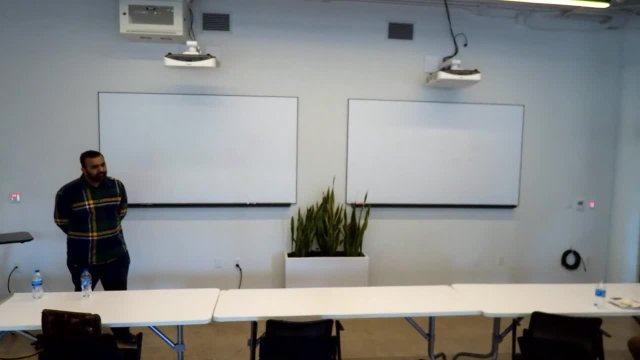 it's like 6.. I think it's like 5 to 10.. Yeah, $8.. Yeah, It's a. I'm just saying it's an old question. Yeah, I was having these discussions at my. No, we were moving. We're basically trying to learn. Quality control is just a validation. Yes, there are failed to validate, but ultimately the solution to that is building quality in the product so it has less problems. But the question again goes to the same thing: How often they should validate, And are there ways to validate more often? 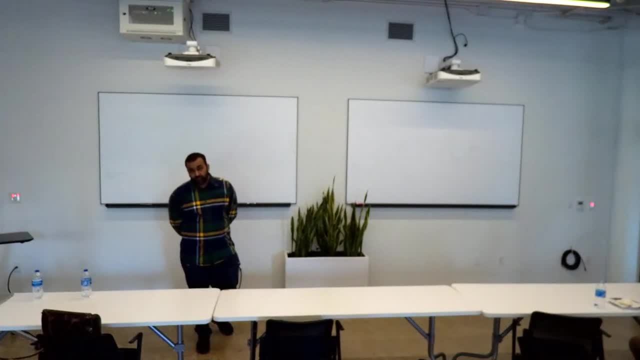 And then, especially, that happened when we were transitioning from waterfall long cycle where you have a development cycle or a large period cycle and you have an agile processor. The problem is you cannot do ways on your continuous development if you don't have 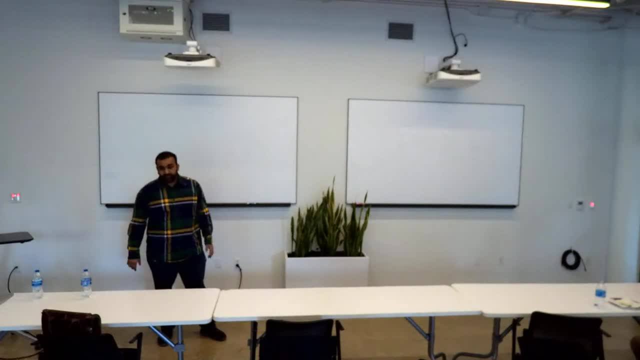 It's not possible. Yeah, Not if you want to move fast. Yeah, You're testing before everything is done. Sure, Right. And so if you make a test and now something changes, that has to be repeated Every time you test. That's if you have manual testing, there's going to be a natural limit function. right That you're not going to be able. so either you have to be comfortable with what will release something or you need to invest in a different mindset. 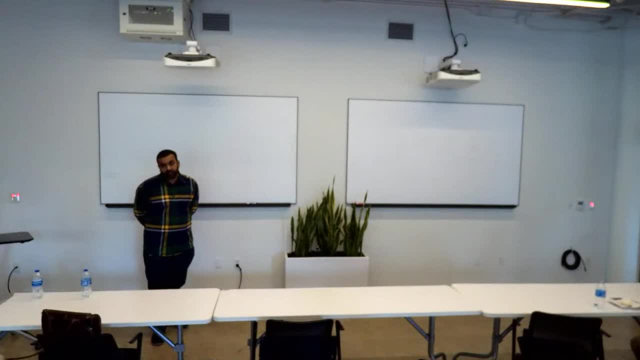 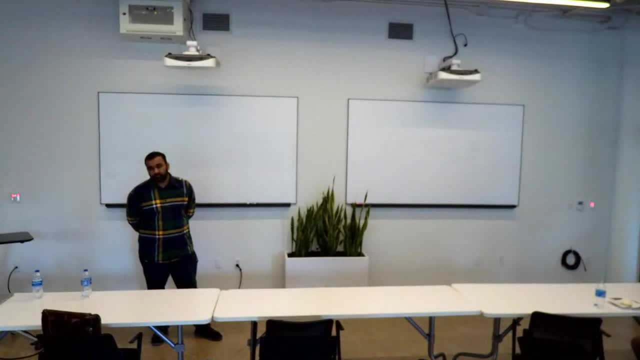 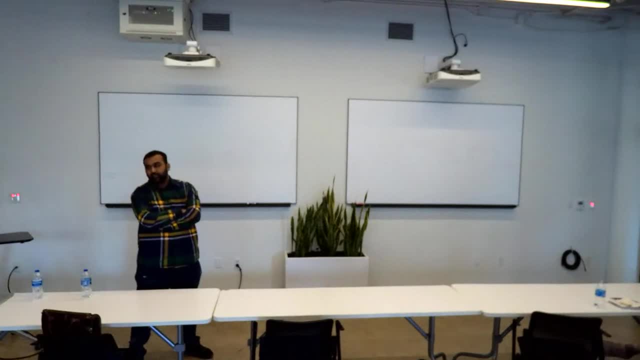 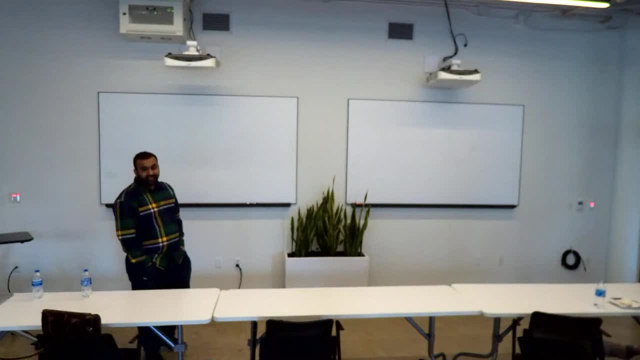 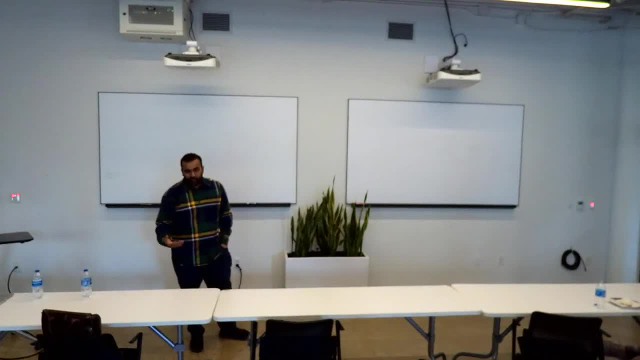 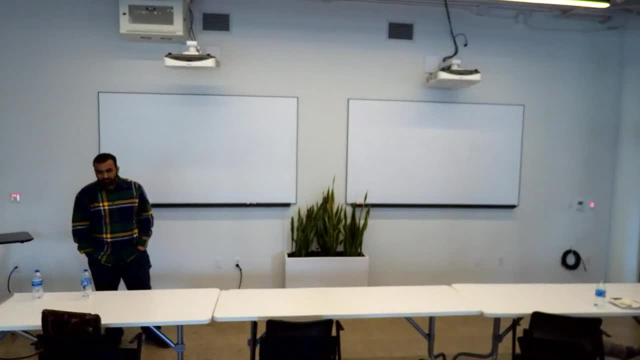 I don't think actually you need to do that. No, I've been not coming into it recently. I'm just calling it back. I'm just coming into it. Yeah, yeah, yeah, that's the way we meet up, Yeah. 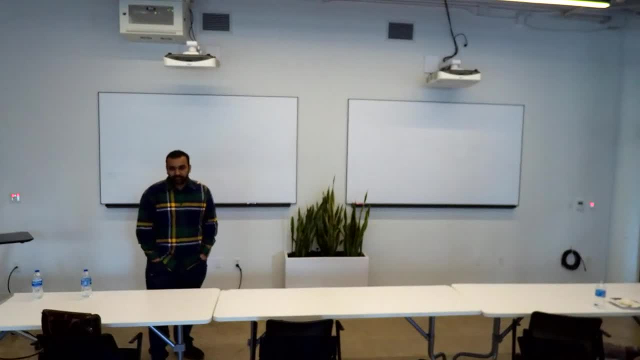 Every day we get to practice, so it's tough, Yeah. so I yeah it's an interesting discussion, but I think the solution I would be pooling same with security. security is the best solution for security control and everything. 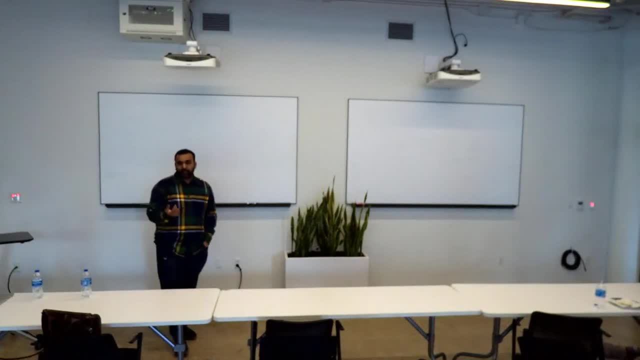 How are they in that control system here? Yeah, and I think that's a subset of problems. Yeah, and I love the security calls. Yeah, They use the whatever tool base to pay for to get things done. Yeah, They don't care about, they do manually versus. 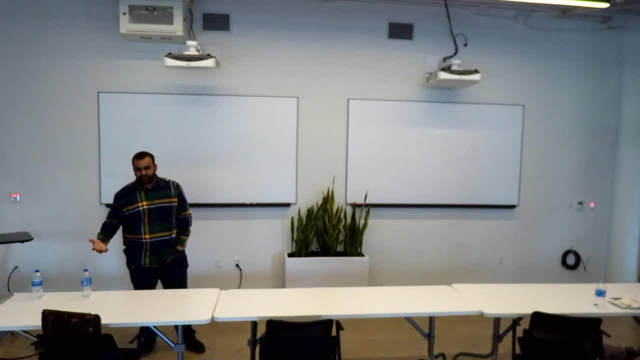 I use whatever They think. this operating system is great. They put their own, They put these are the scanners they want to put in. but they use the tool and get things done. Yeah, but the problem that's happening is the old, old time UA problem. 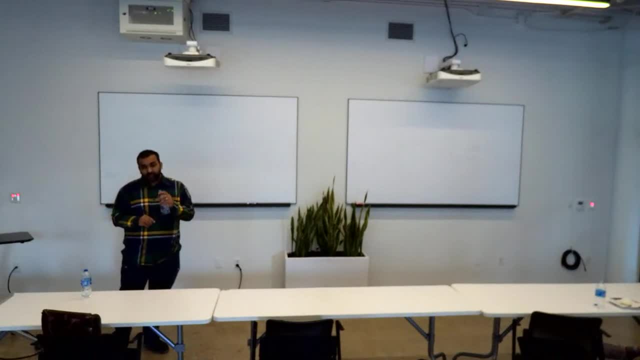 where there's control over the fence, where there's two fighting each other, that team is doing things. Now you have, you know, a developer that goes and uses something and does something wrong, and then it's security tested, you know. 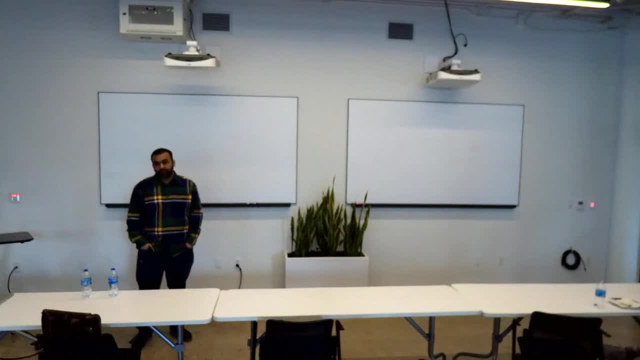 down, further down the process, and then they use a scanner and then a bug comes in and they're not in contact. So it's the same fight, right? Like my role is to help with the security problem. Like: is it applicable? is it not applicable? 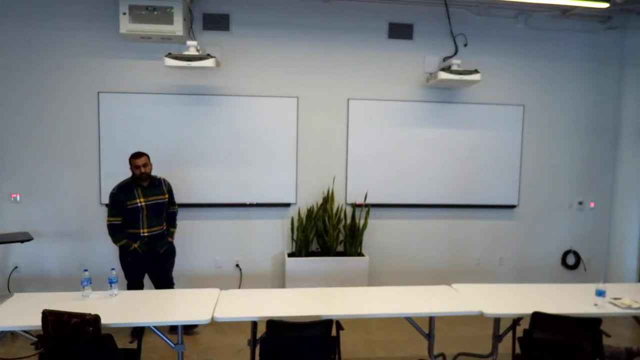 is it a threat vulnerability? So the same friction is happening and I think the same solution applies. These are just what can I say? It's like watch out. you know it's the same thing, but it's the same. 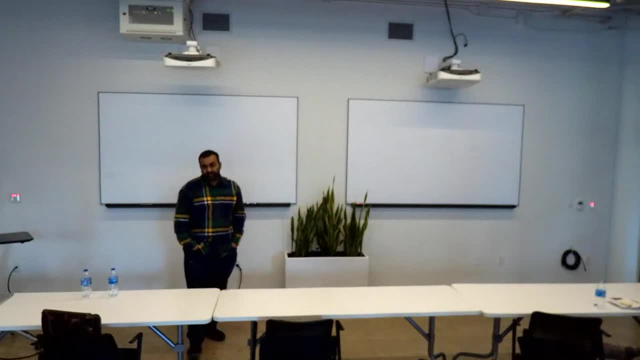 Because you have silos in everything and you have goals that are not holistic. right, My goal is to find as many bugs as I can, So that's my problem, you know, like you said. And the other one is I'm going to check this out. 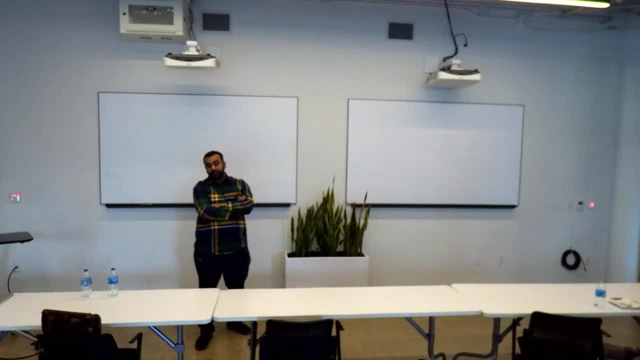 That is the main thing that you have in mind when I develop context. you know the main context. Yes, Because you know if you have a lot of bugs and you have a lot of problems and you have a lot of problems. 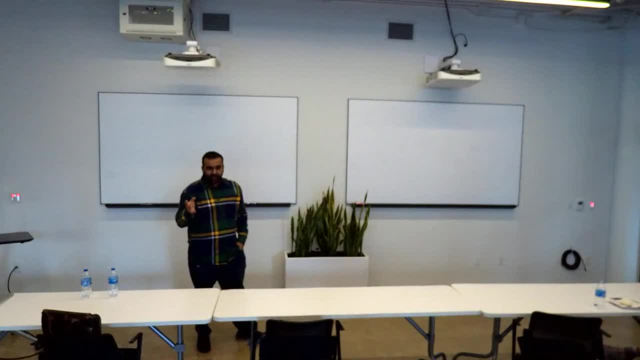 and you have a lot of problems and you have to read them and you have to think about how you can help solve the problem. Yeah, So how to solve the problem? I'll take that question. Like I said, the first context was missing here. 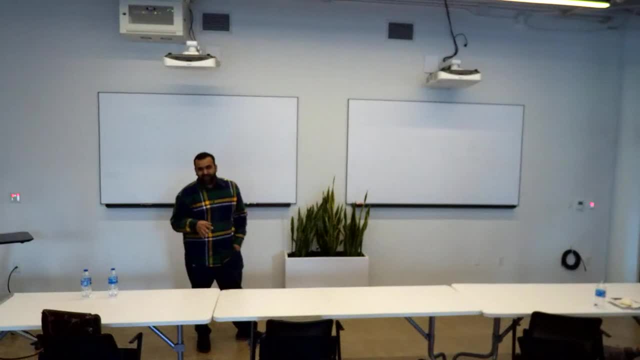 because it is a practical mailbox product if you need 100%. there are a lot of bug cases and then it goes into: Hey, what is the bug? Where is the bug? There's your problem called What happened? What we brought is. 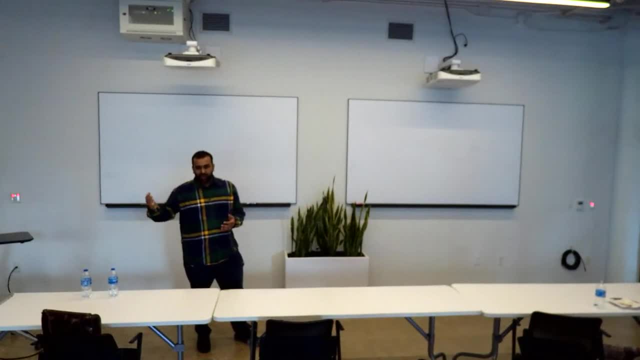 it is a waste of time All the time. that's what I was like. okay, it must be automated, but also providing the context as much as possible through the developer: what happened, why happened, at what step happened, so they can have a correlation. 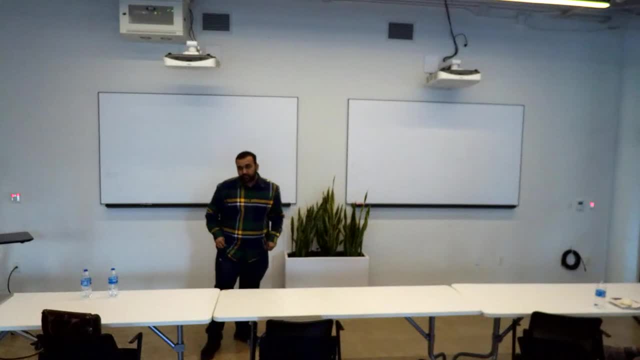 and then they can attack them. That's why ultimately, in a very mature evolution of that, all that responsibility is some kind of producing, And the producer is just using more advanced tools to make their job shift left, so they can know these things early. 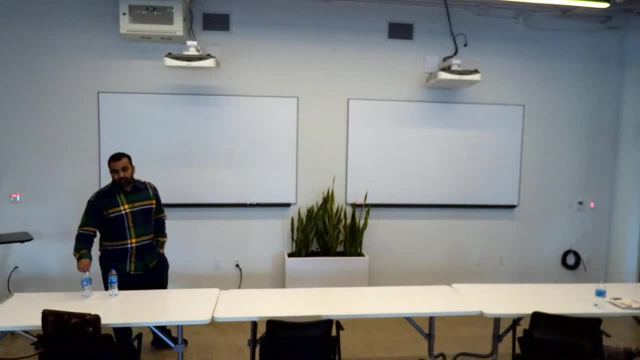 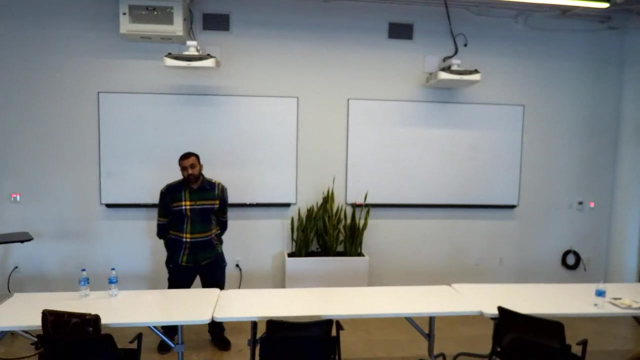 So when I in my ID, I'm about to push a full request, then it tells me static analysis of the code There's some SQL injection problem, There's some SQL independence, whatever it may be. So now they are responsible for fixing it. They're just getting feedback loops much sooner than one month later, when it's I don't know where, Somebody said, hey, there's a bug. Now you lost all the content. Now you've wasted 100 times more effort to figure out what went wrong. No, but that's what I'm saying. That's how continuous integration. the goal was exactly to reduce those feedback loops, Just reduce them. The more you integrate, the sooner these problems arrive at your footstep. If you wait too long for integration, you only get notice of the problem further away. 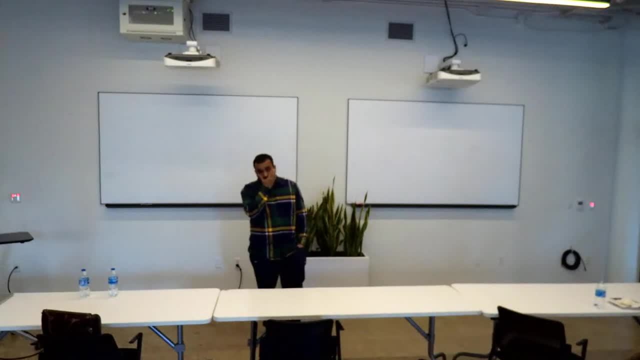 And the typical example: you take a shower. Imagine that every time you rotate your water cold, it takes two minutes. Try having a shower that way. It's really hard. It's really hard. You have to wait literally, say, a minute. 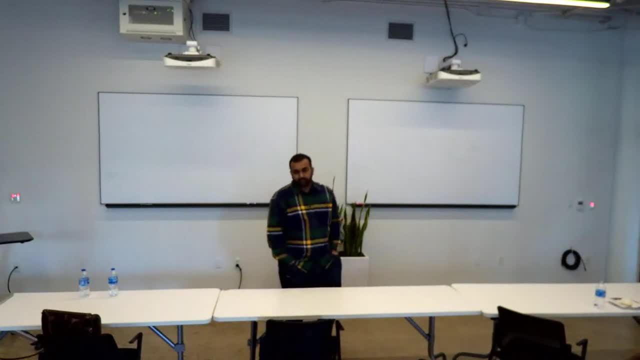 So the whole point, the whole solution is the same. So you have the context of the information. As I'm developing, I can know immediately. That's why you want to put it in production as soon as possible, right? Because then you're going to get those sequels. Yeah, it must be like, as you mentioned, you linked those two different ways. Whenever you compile, I mean It should be as fast as that label. That's the whole label thing And that's why the sprints have reduced. 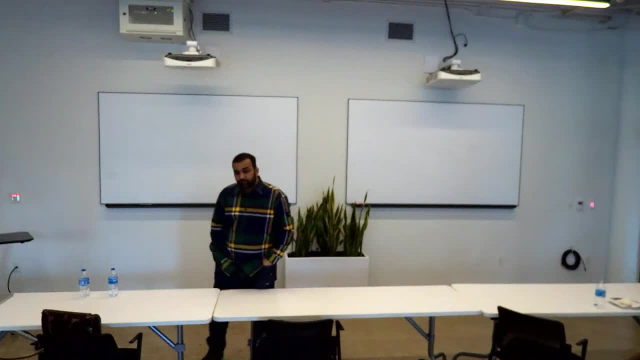 And that's why you want to. If you want to move faster, you want to reduce the size so that you can push that faster. So you have those. Ideally, that feature, that time. But it's hard Because time is a scale right. If your STLC for one feature requires 29 days, then you can't do that. So that's the only solution for that. The maturity is true And it's platform engineering to make that. And so when I was developing, even in developers, when you do feature development, eventually your product gets complicated. You may need a business tool. then it's platform engineering, So that's not related to the feature right. But you need something that's going to help you move faster, Otherwise your feature development has to stop completely while you go develop some. 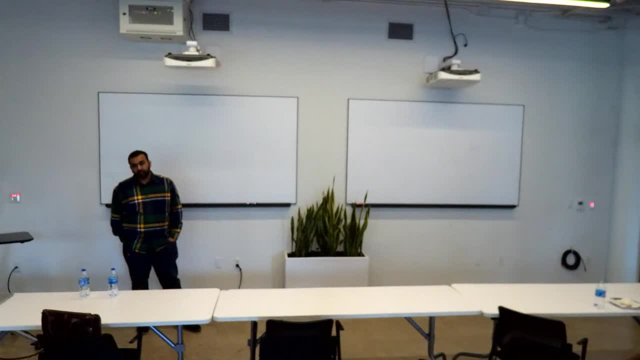 plumbing to do the part. So the idea of the platform engineering is to support that. Now, that name is just. the platform is just gotten bigger and bigger and bigger. But I think it's the same. What I was trying to say is the same thing over and over, just touching more idols of. 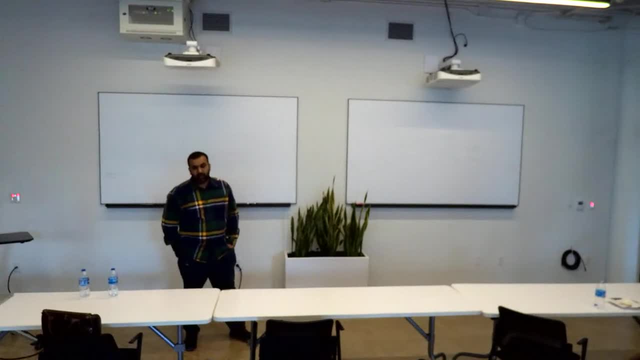 that tool, experience of what it takes to do that. Yeah, Yeah, I think I got your point. So the concept is the same, but with the time cost, Yes, With the AI coming into play wherever it is happening, I wouldn't say that we have. 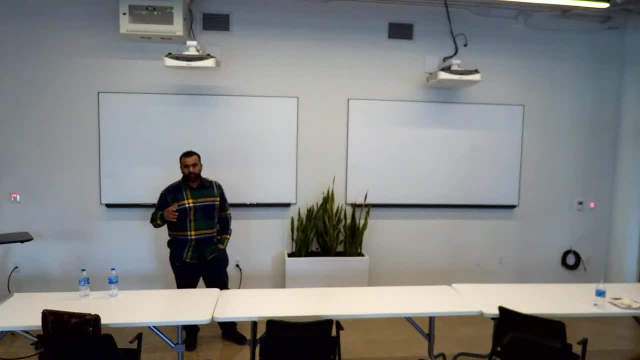 But with the AI and the tool, yeah, it is about the maturity only where it is helping to. in two cases: the tool is getting stronger, awareness is getting better and adoption is getting better. Those are the things that helps us to go towards the future. 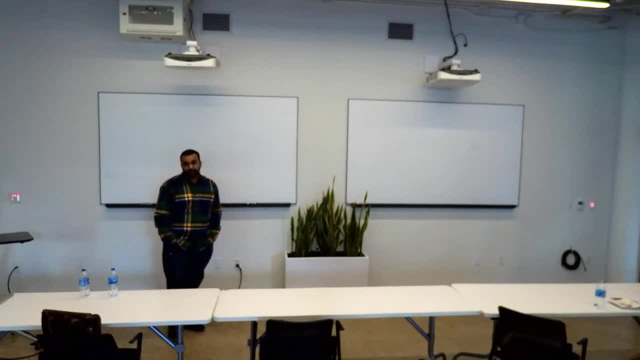 Yeah. And then there's shipwrecking, Yeah, Shipwrecking, Which is why we have the interaction factors Mm-hmm When we do this. Oh, so, you, Yeah, So we have a lot of different things that we can do in the future. 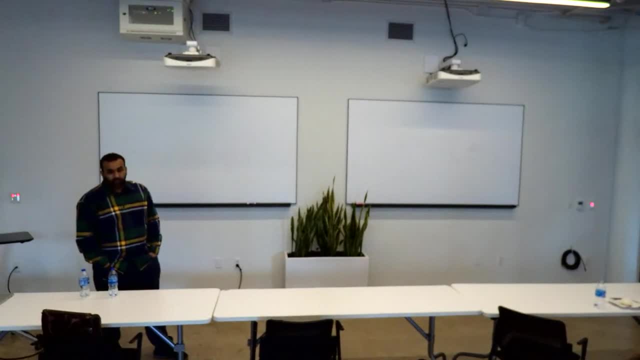 Yeah, Yeah, Yeah. So I think the first one is what we call like: what's the Mm-hmm? So is that all in the scope of your idea pretty much, Or is it a big way of? Well, I mentioned that last, but 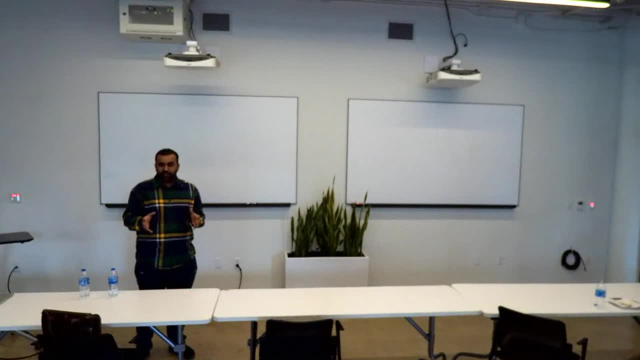 Yeah, Yeah. So it is about how this thing plays a role and how this stuff can play a role in the before and after. So this is the first topic for the in-process discussion. but we want to touch from the requirements through the like development cases, how AI and in real time can be used. 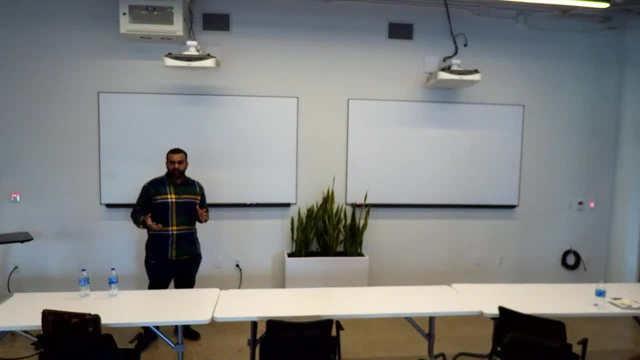 to do these things. Yeah, Yeah, And we can have from the to the development cities, Yeah, And they can do the design and then do the and all the way to all the way, And using this and get the feedback from the and, more of all, the data and. 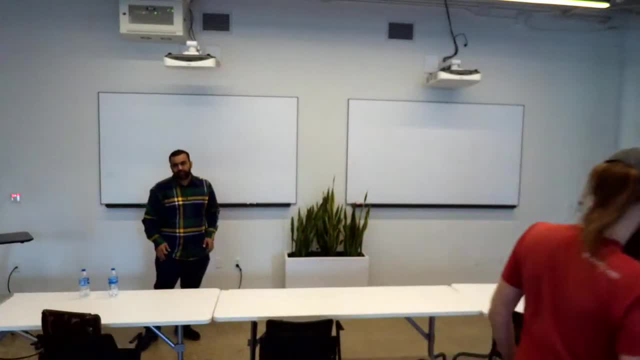 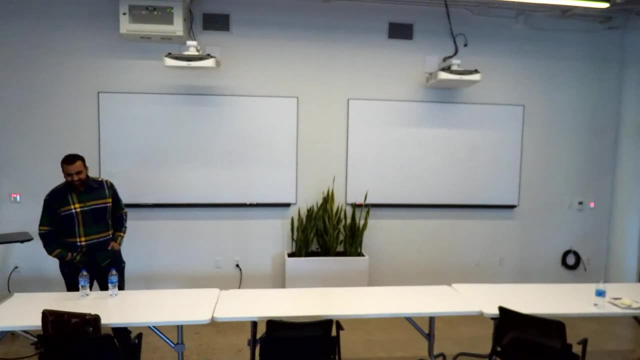 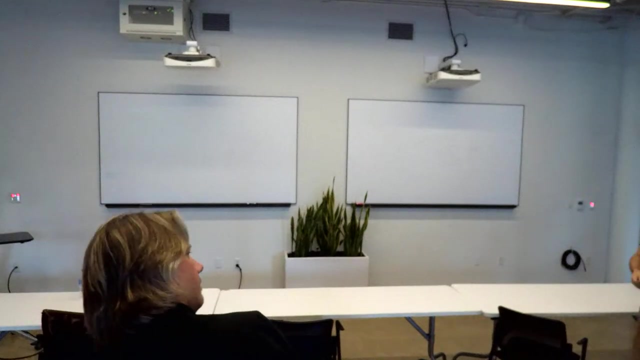 and all the OK Appreciate it. Yeah, Yeah, Thank you very much. Thank you, Yeah, All right, Thank you, Yeah, Yeah. Yeah, Which company do you work for? It's Caringfree, It's a non-profit. 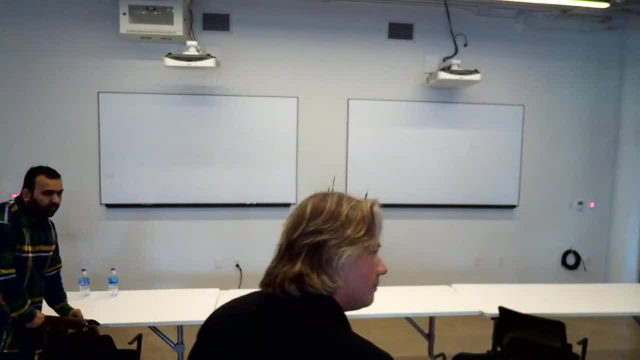 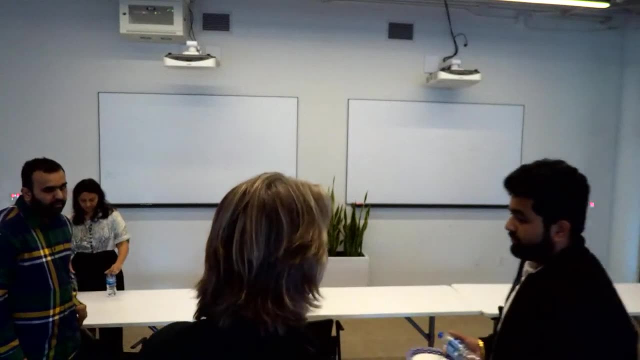 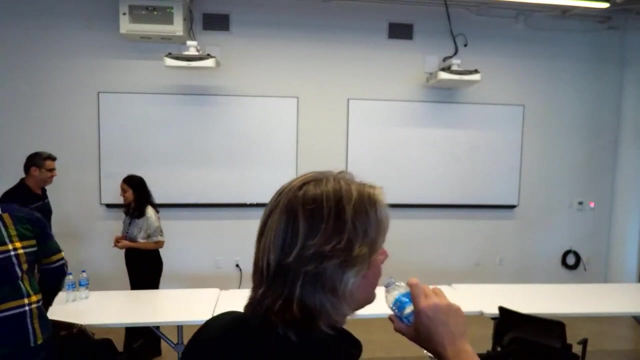 What about your company? are you in? Yeah, I go, I go. What do they do? It's like John Deere. I'm always amazed at the level of innovation that those companies have: The device level, IoT, sophisticated stuff. 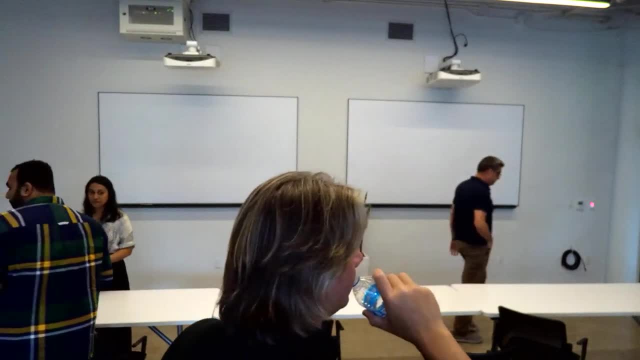 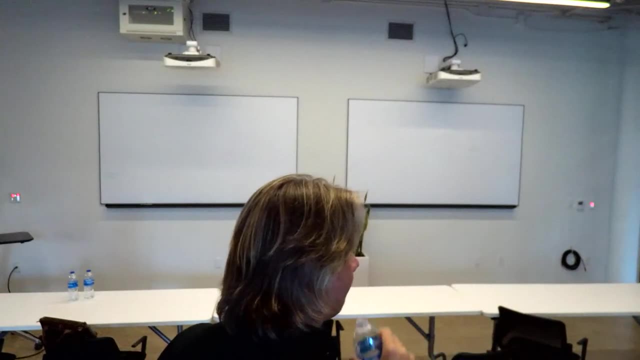 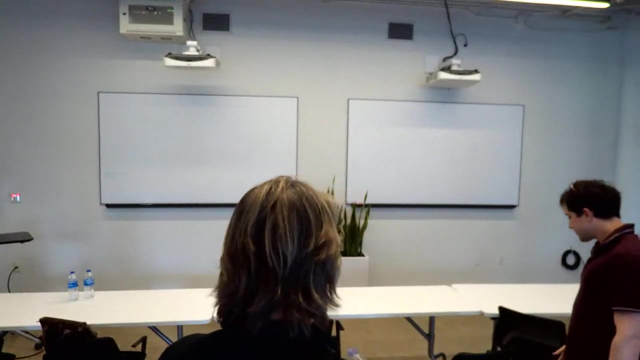 I met a guy that actually used to be in the media. He worked for Africa. He does some pretty cool stuff. Yeah, it's like there are fewer farmers than ever and the reason is technology. I was ever surprised by it. It's quite technology heavy. 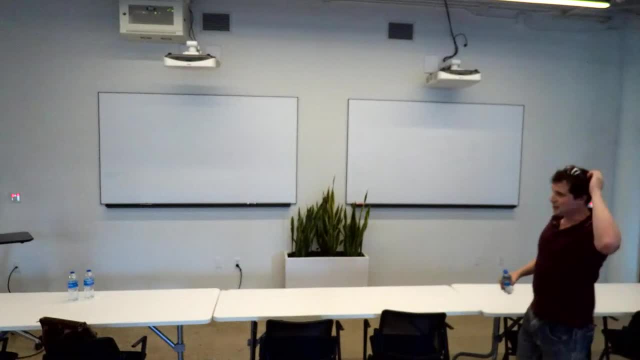 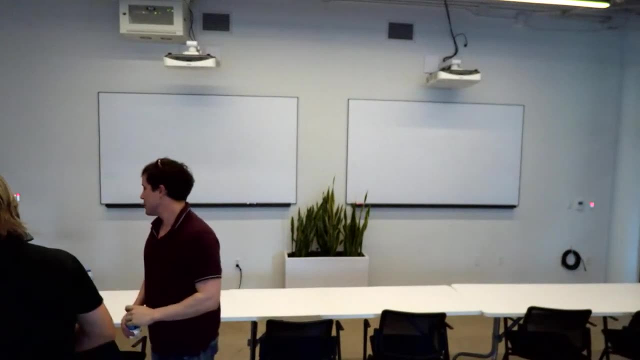 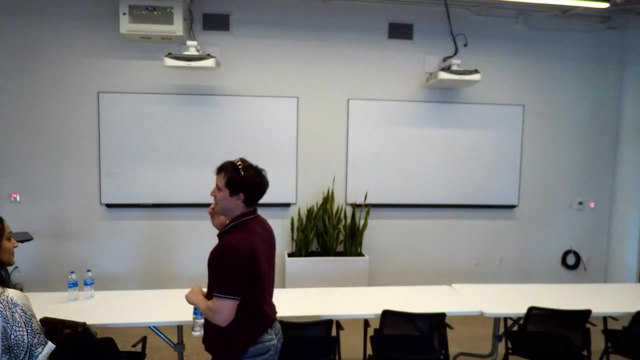 More than people realize. Well, technology is. no one wants to be a farmer anymore. Oh yeah, Karina, I did have one more question. This year you're putting on Lighthouse, because even Facebook, when I go to Facebookcom, Lighthouse, I get 72.. 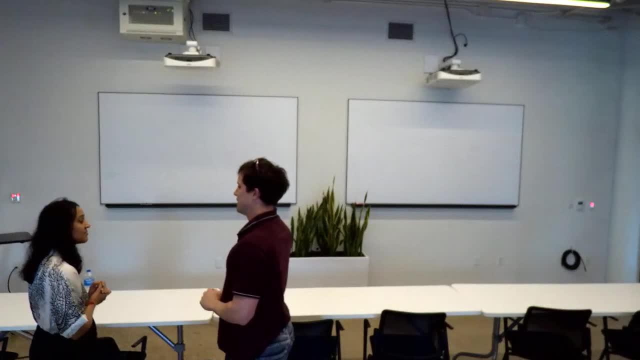 So do you think Lighthouse is really useful? Yeah, Yeah, sure, Oh, hey. so you're like young guys just use Lighthouse. Yeah, I should go. Yeah, technically I don't know. So, Lighthouse, you think it's good or no? 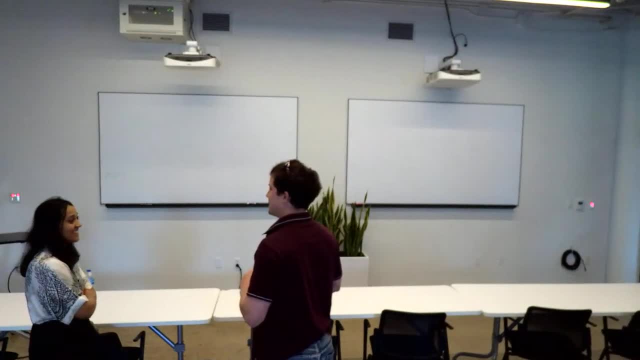 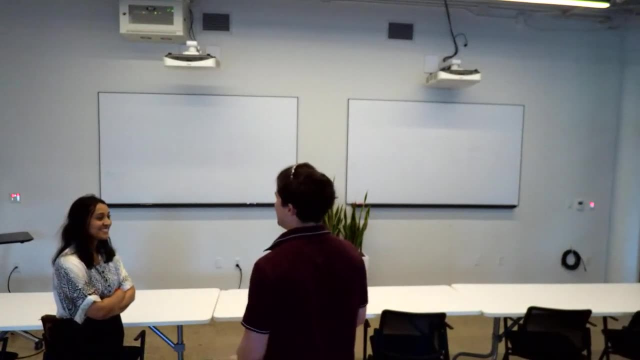 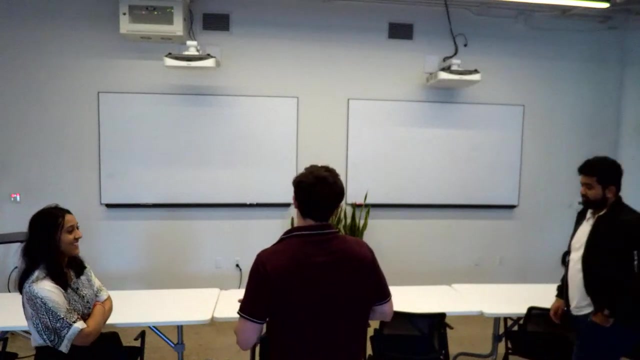 Do you think it's good or no? It's not good. Maybe they can work with it. Okay, that's good. So how can Facebook have a low score? Or YouTubecom? it's not as perfect. So it's like if I can get a 100, then maybe YouTube and Meta can do it. 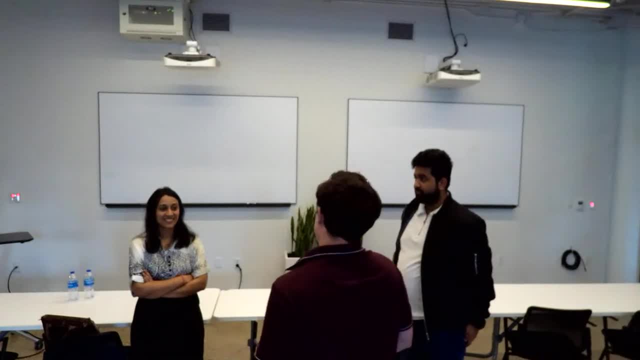 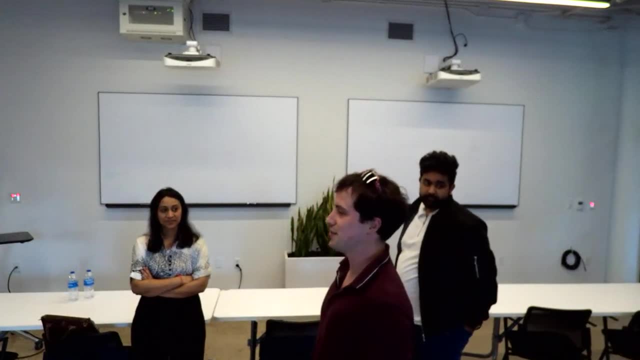 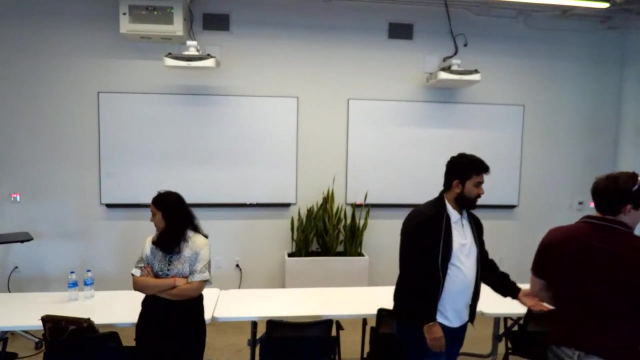 But they don't. So Hulu is very cool. All right, guys, Wave. yeah, that's really cool, Awesome, Yeah, nice. What was your name? It's Julian. Do we have to make this video at home? Yeah, I'll take one. 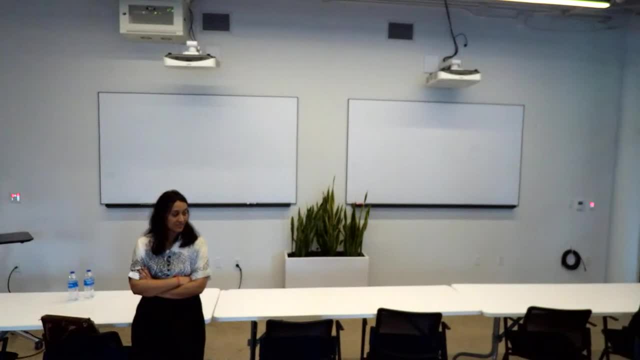 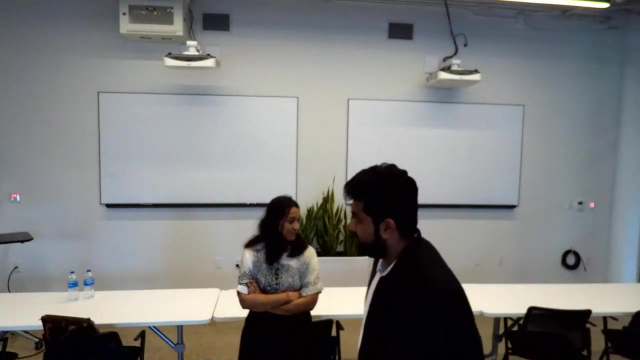 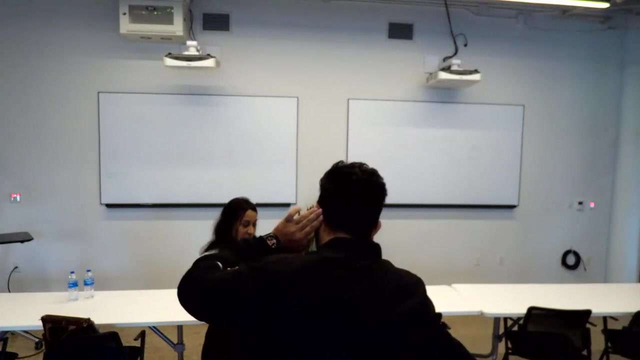 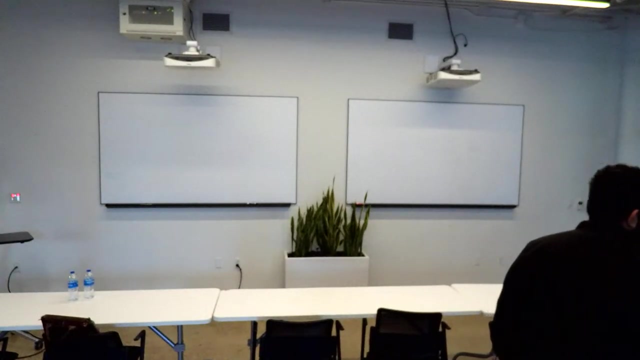 Okay, Yeah, Maybe I'll get this one All right, Thank you. See you in a minute, Excuse me. Nice to meet you all, You too. 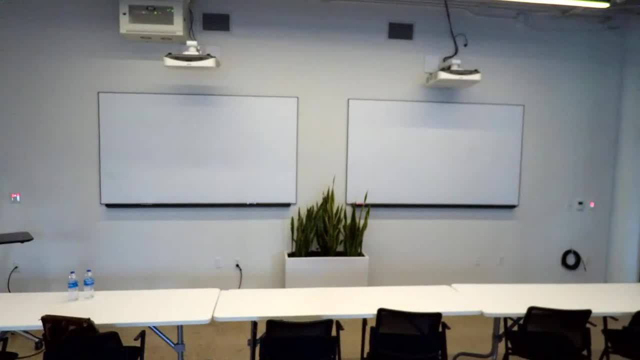 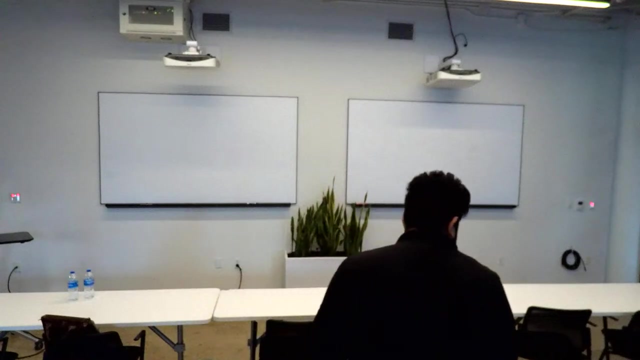 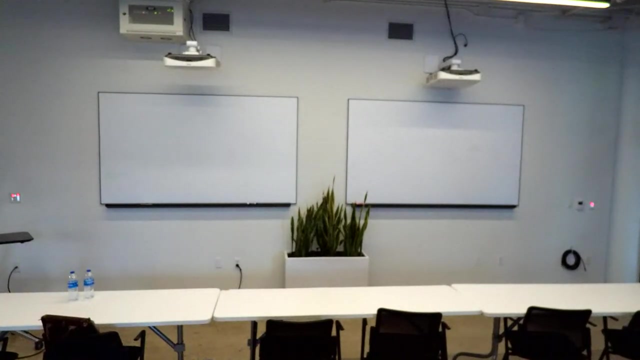 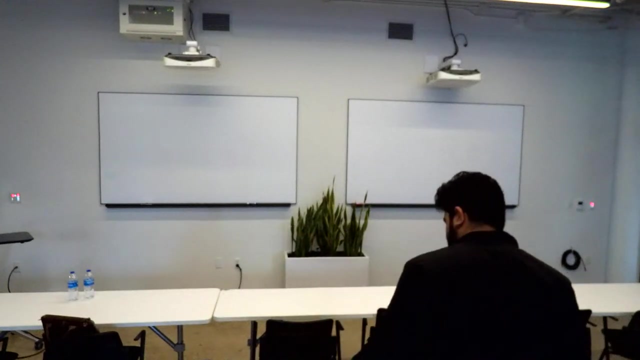 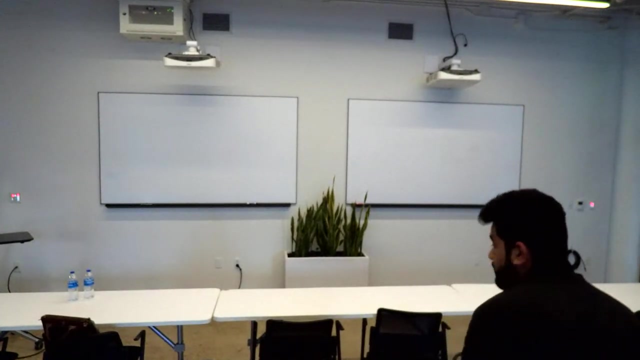 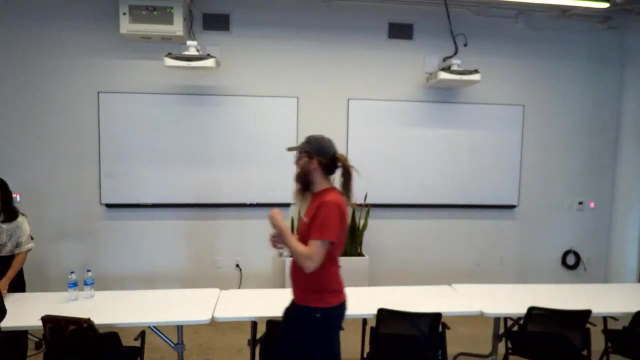 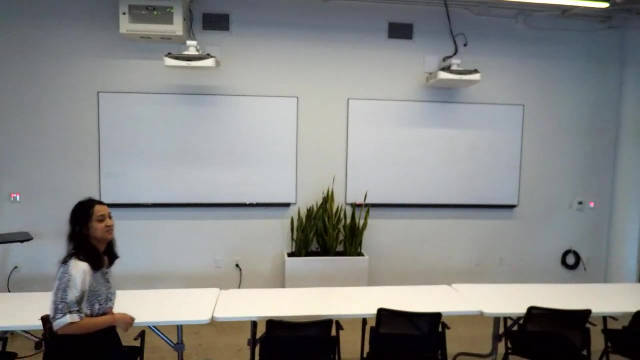 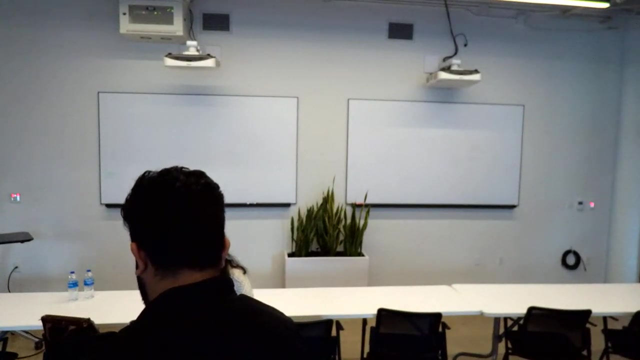 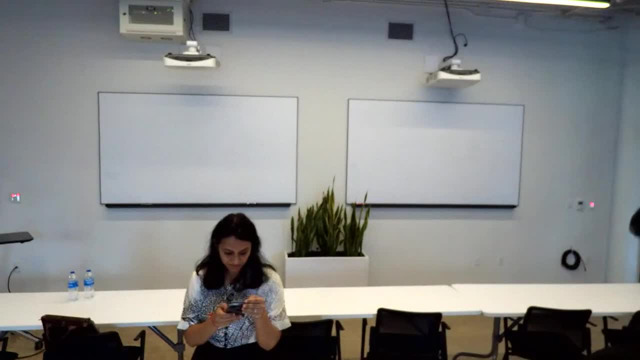 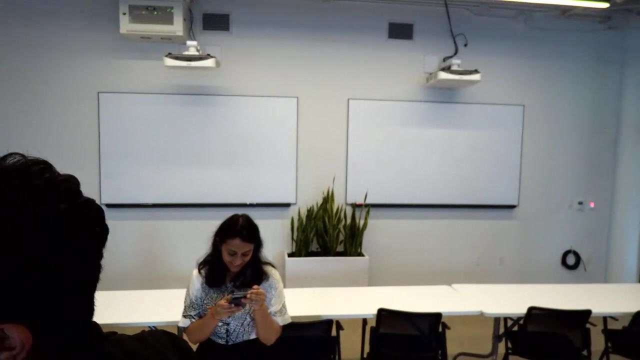 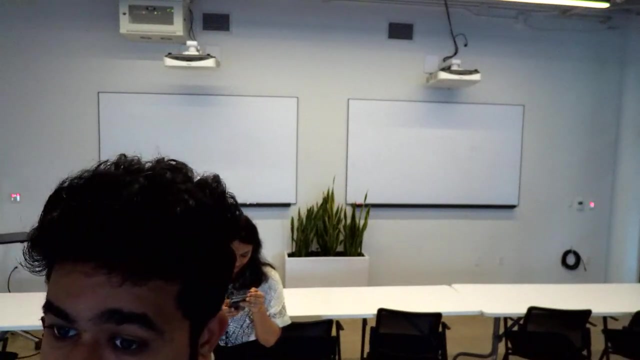 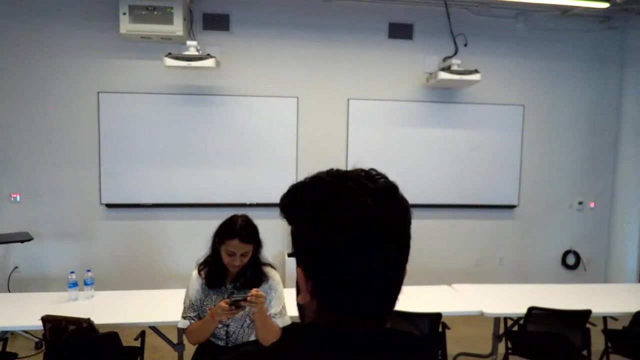 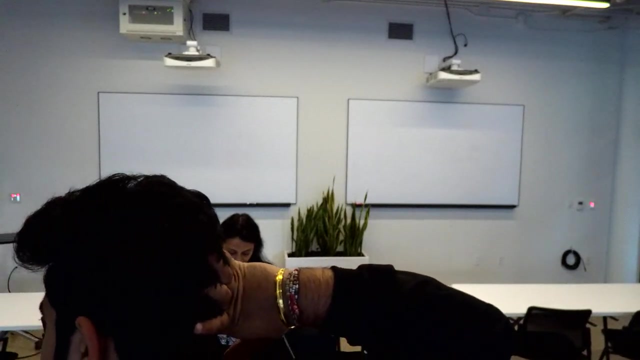 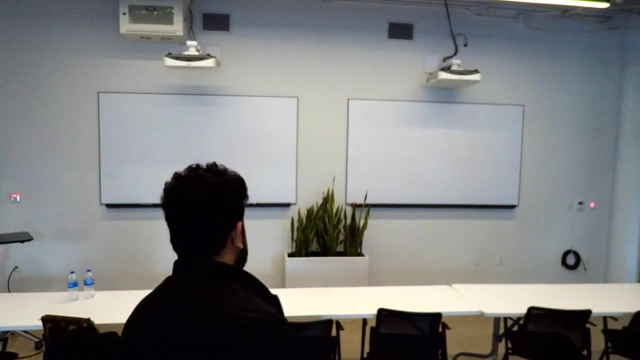 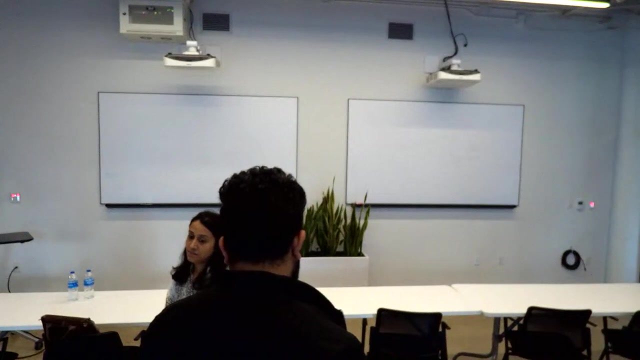 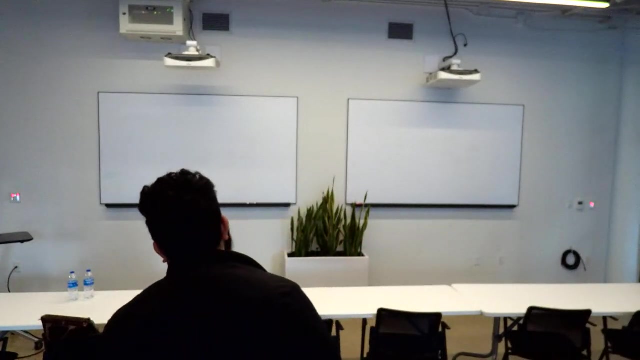 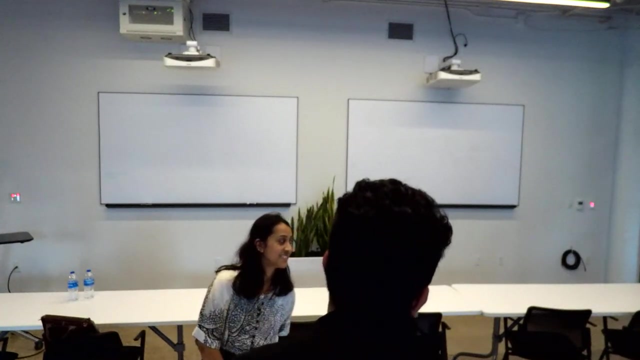 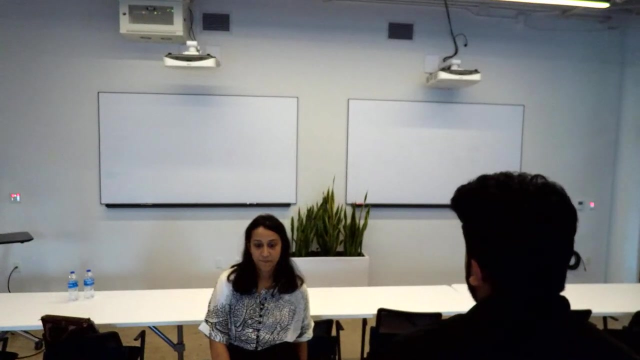 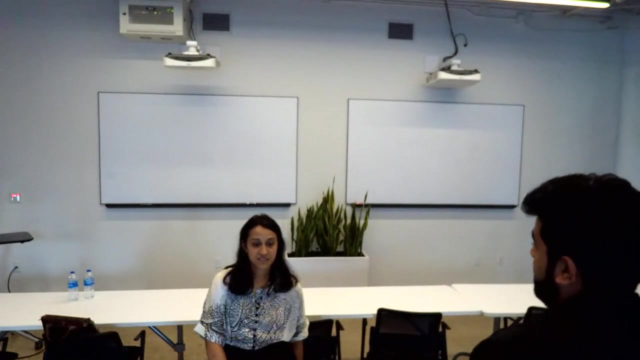 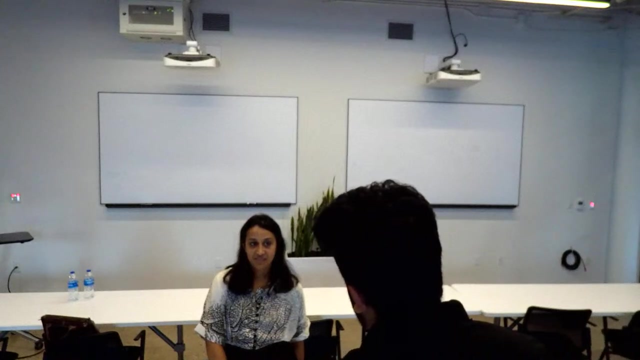 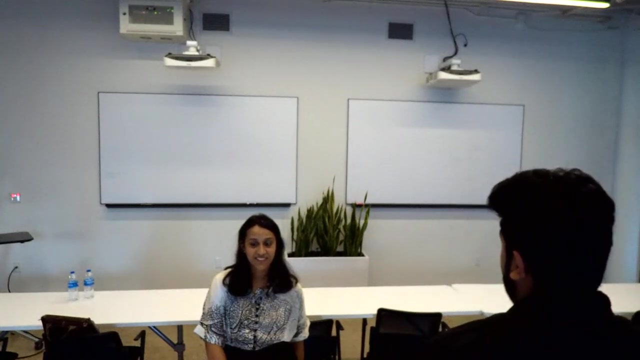 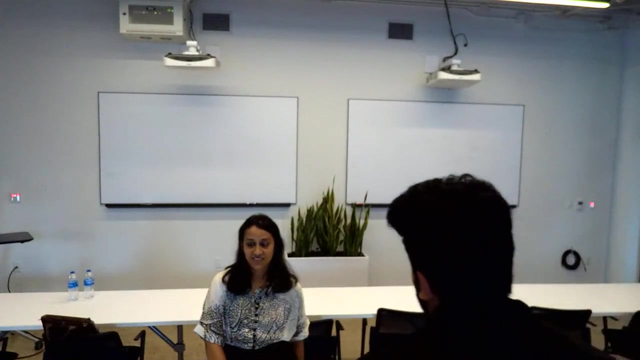 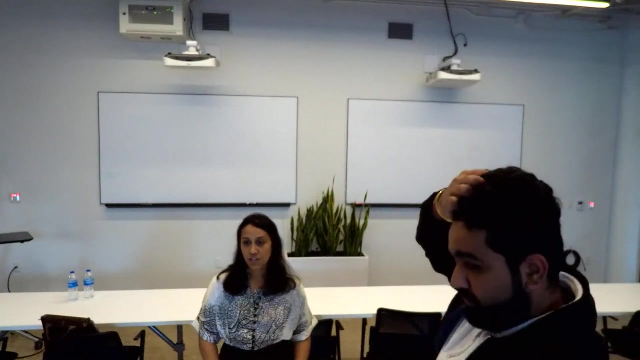 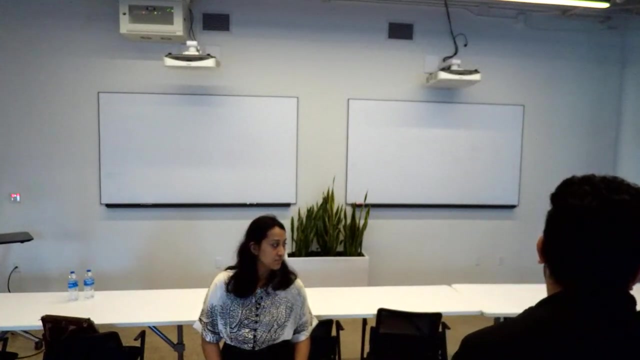 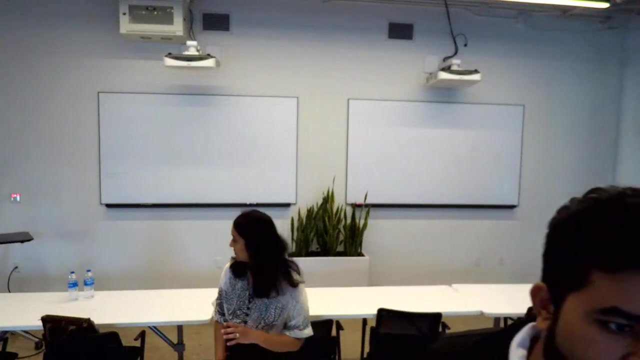 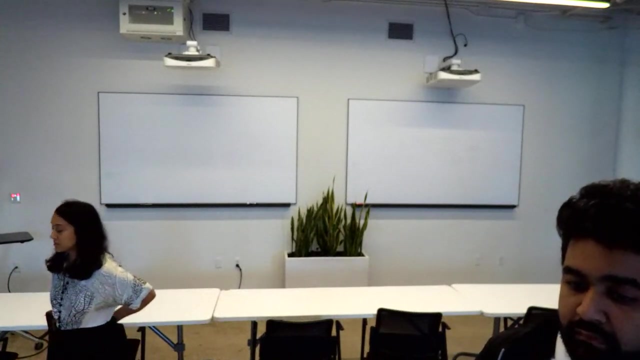 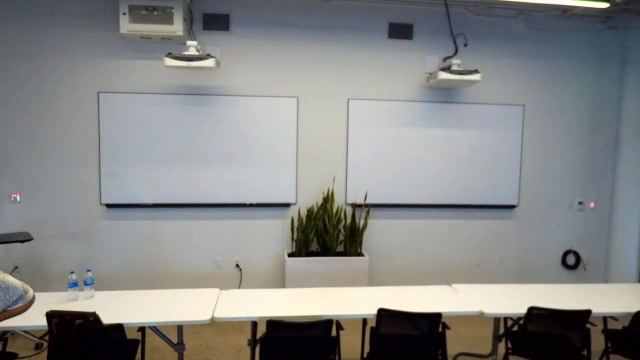 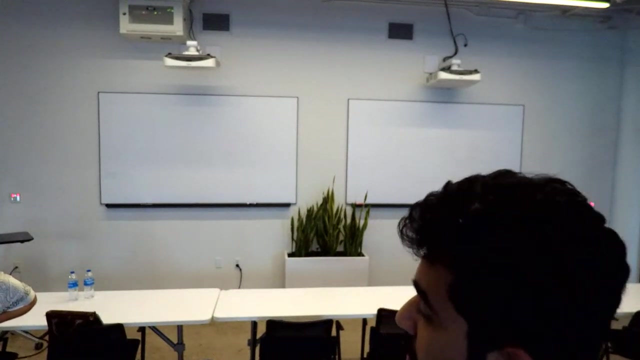 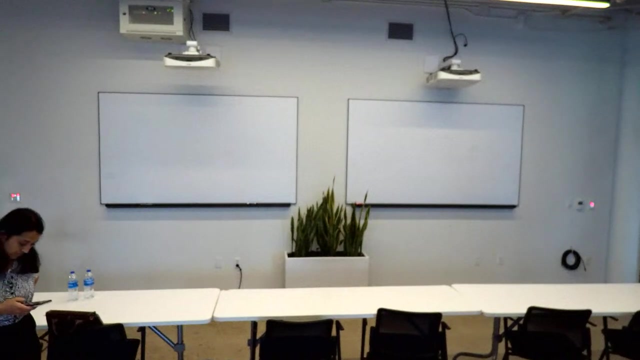 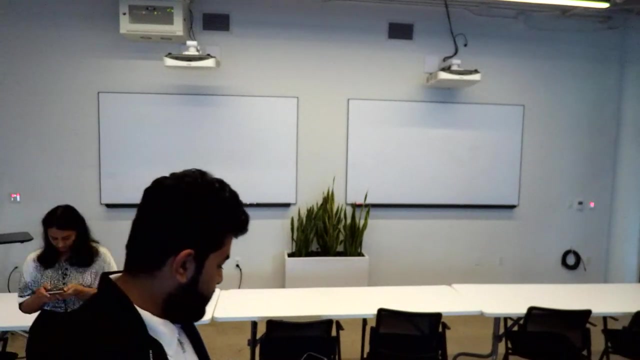